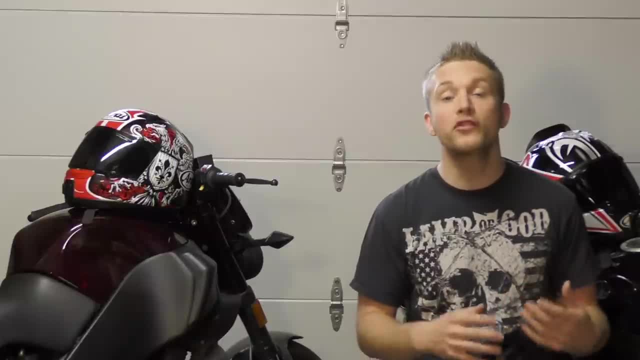 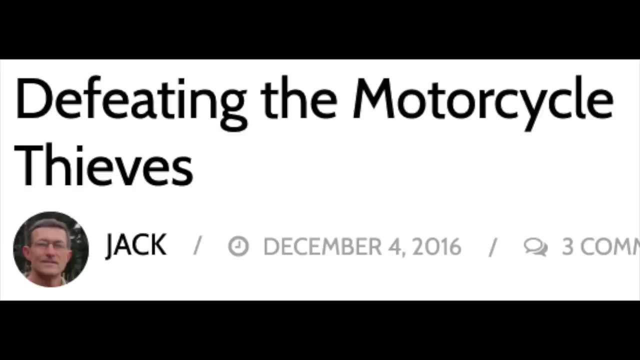 to understand the how and why of motorcycle theft in order to make the most effective decisions to reduce the likelihood of having your bike stolen Enjoy. Like seemingly every popular motorcycle topic, there are tons of anecdotal information and recommendations out there about motorcycle theft. A cynical person might even start to 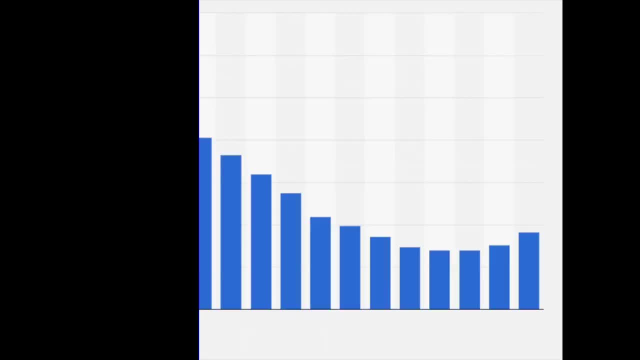 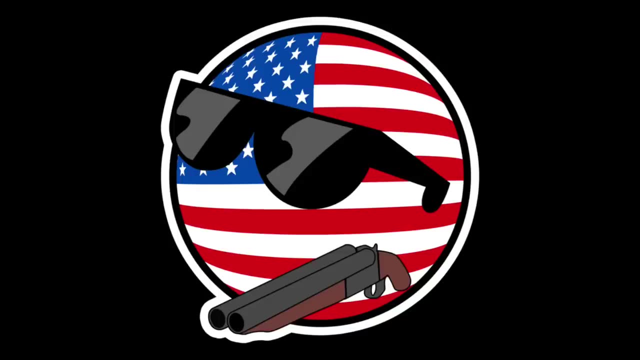 think that many of these videos are just created to try and sell you something. So let's first look at some objective statistics to get a baseline of how prominent it is and see if we can tease out any patterns or trends. I'm going to use the US as the model for this. 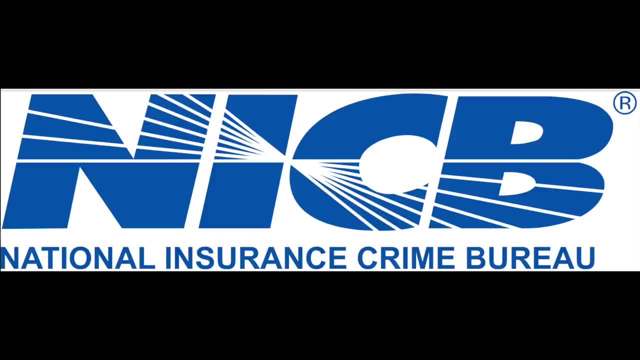 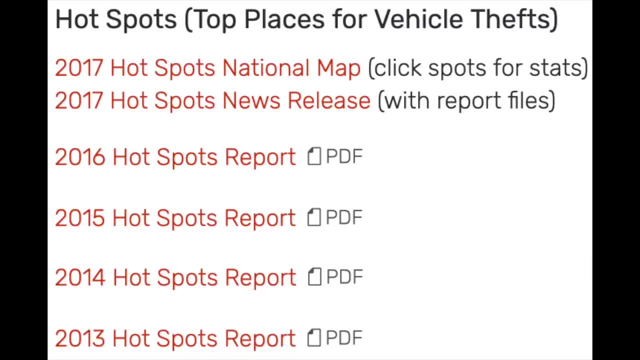 information, But I think we'll find the takeaways are pretty simple. The National Insurance Crime Bureau, which is a non-profit created by the insurance industry to address insurance-related crime, does a decent job of aggregating motorcycle theft statistics in the United States yearly. In 2017, there was over 44,000 motorcycle thefts. 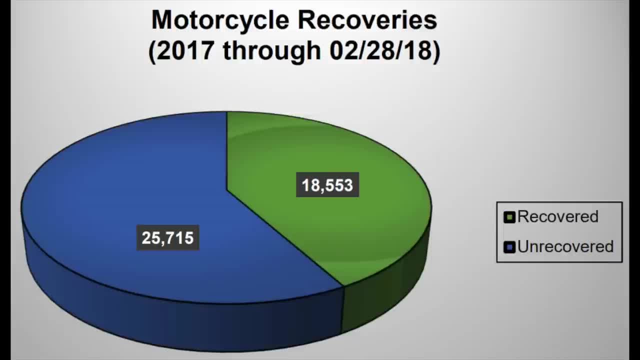 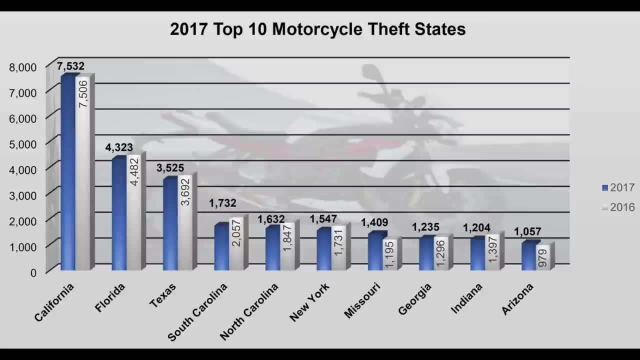 with a recovery rate of 42%. That's right. If your bike's stolen, there's less than a coin flip chance you'll ever see it again. In the US, the top states for theft are California, Florida and Texas, with the rest trailing off quite a bit. This isn't really. 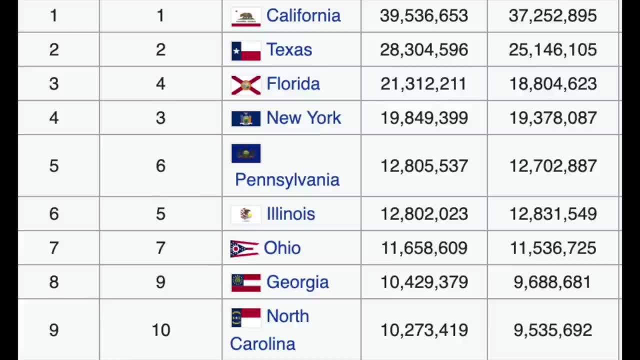 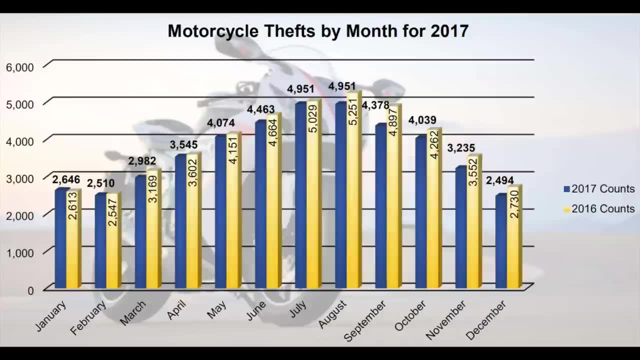 surprising, though, because California, Florida and Texas are the states with the highest populations, So it makes sense that they would have the most motorcycles, and so the most motorcycle theft. Motorcycle thefts are increased in states with warmer climates, and there's 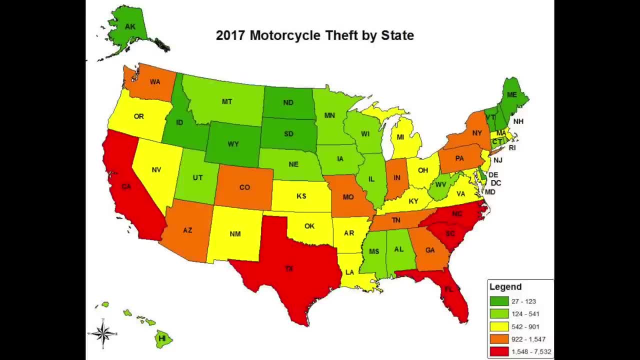 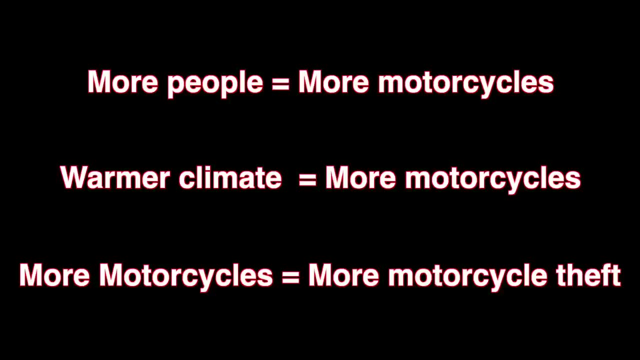 a clear trend that thefts increase in summer months In the trailing states. there seems to be a correlation in theft between high populations and how warm the climate is in those states. It seems obvious to me that more people ride motorcycles when the weather is warmer, so there are more bikes out on the road visible and accessible for potential. 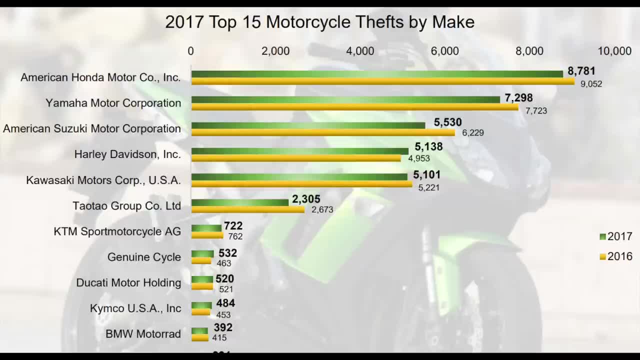 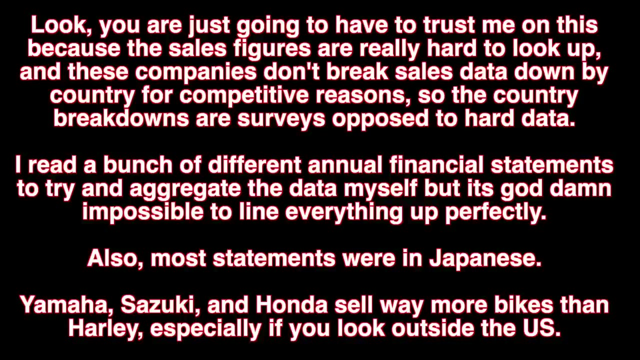 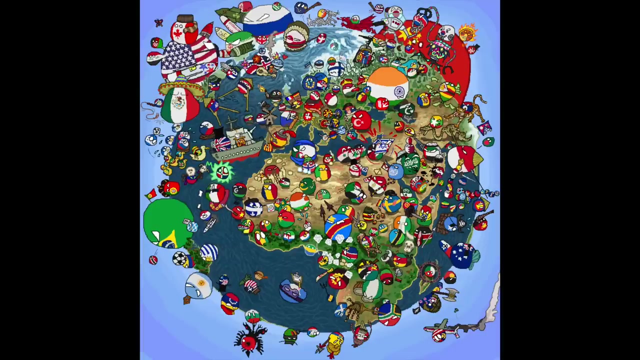 thieves, which increases thefts As far as which makes and models are stolen. Asian manufacturers- Honda, Yamaha, Kawasaki, Suzuki- lead the way. The only conclusion I think you can take away from these statistics are that motorcycle thefts aren't really based on where you live or what you ride, but what's available in. 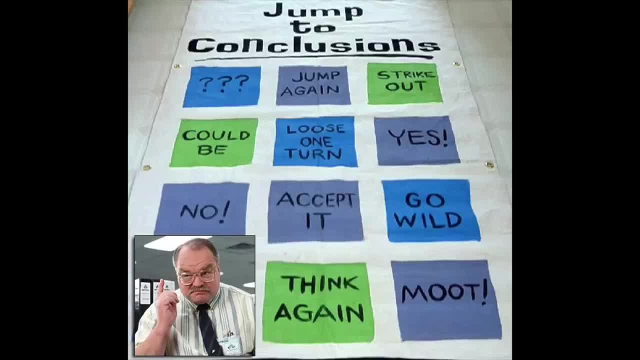 the wild for thieves to take. This supports the conclusion of a few studies on motorcycle theft, which indicate that it's most often a crime of opportunity. Just to define terms a bit, the definition I'm using for a crime of opportunity is that would-be thieves are more likely to steal a motorcycle. 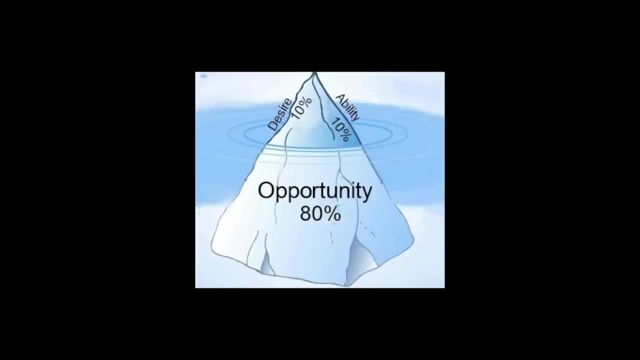 and more likely to steal a motorcycle than to steal a motorcycle and more likely to steal a motorcycle. The reason for this is that most thieves make a simple risk-reward assessment when deciding what bikes to steal, and that increasing the risk cost or reducing the opportunity are 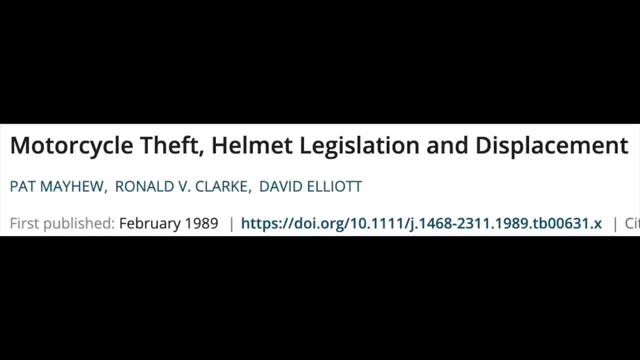 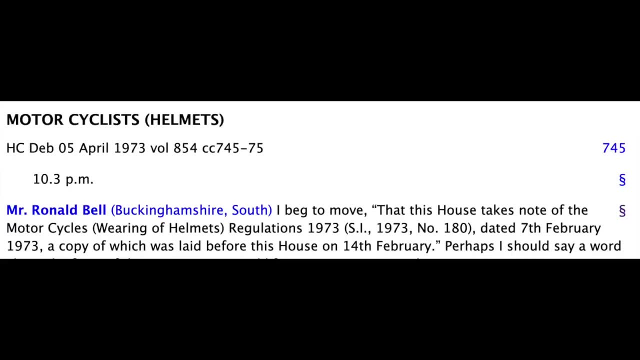 the best ways to combat this type of theft. Let me give you an example of where a simple increase in risk for thieves created a dramatic difference in combating motorcycle theft. A study from 1989 in Germany found that after implementing a helmet law for motorcycles, 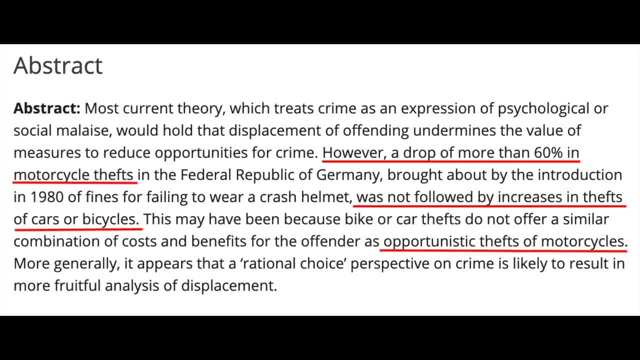 motorcycle theft dropped 60% by 1989, while car and bicycle thefts did not increase. This is because the opportunity cost for motorcycle theft increased, as would-be thieves could no longer roll up to a motorcycle without a helmet and take off. 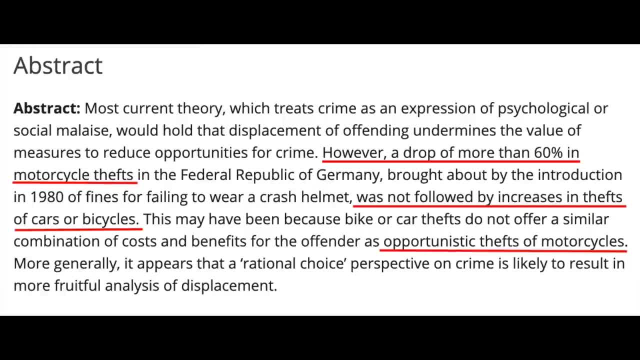 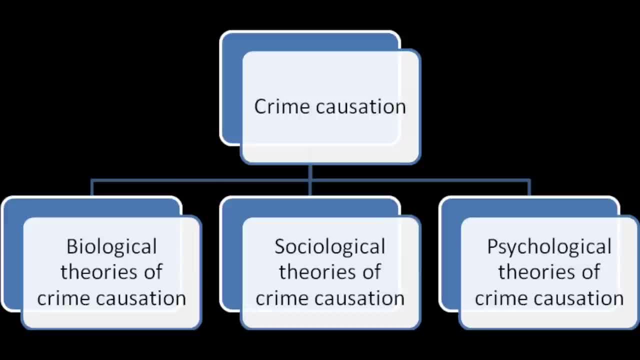 This reduced overall theft because the risk cost for cars and bicycles stayed the same. Motorcycles were just a much easier score, which is why thieves prioritized them. Actually, there's been a variety of studies around the theory that most crimes are crimes of opportunity in some way, but it's a contested and debated theory. 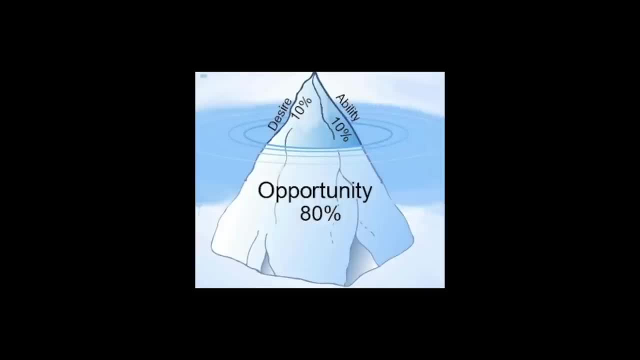 In the case of motorcycles, though I believe assuming this theory holds true for the majority of motorcycle theft leads to making the most effective decisions around prevention. One more thing to review before we get into the specifics of prevention: How are most bike thefts pulled off? 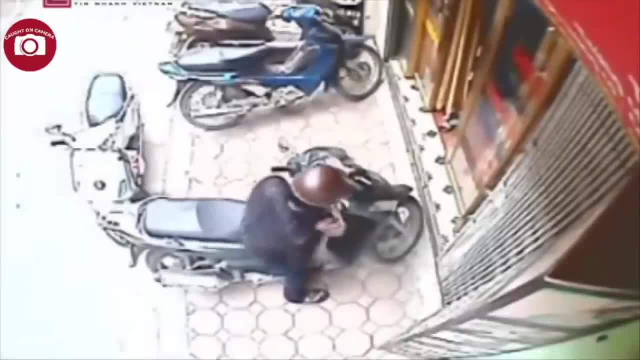 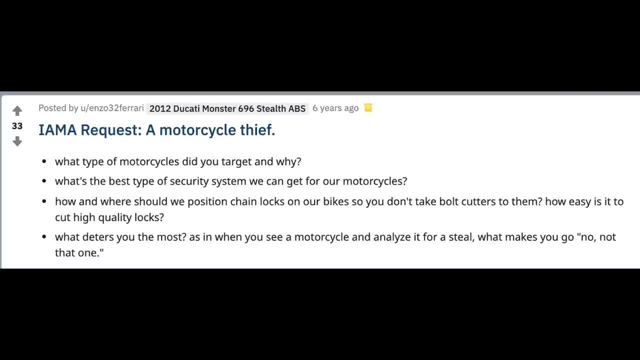 It's hard to get statistics for the how behind motorcycle theft, but if you look at the statistics for the how behind thefts, we have to rely a bit on anecdotes. However, it does seem that the more credible of these former bike burglars and chop shop 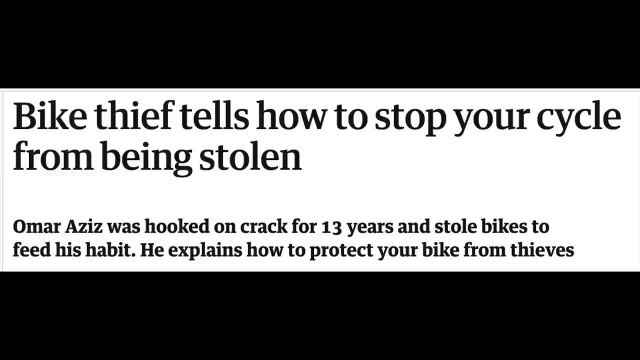 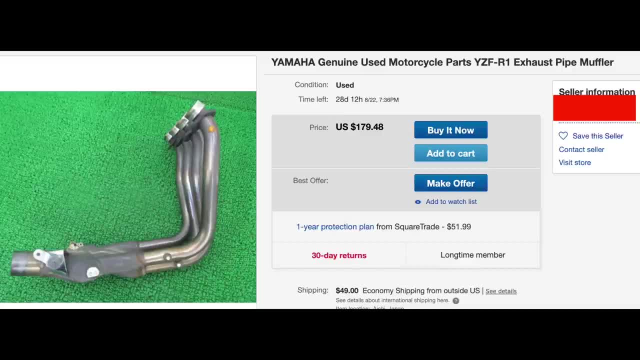 owners describe common specifics around the methods and tools that paint a fairly detailed picture. The objective of the average bike nabber is either to sell the bike to a less scrupulous bike shop that will part the bike out, focusing on selling components without traceable serial. 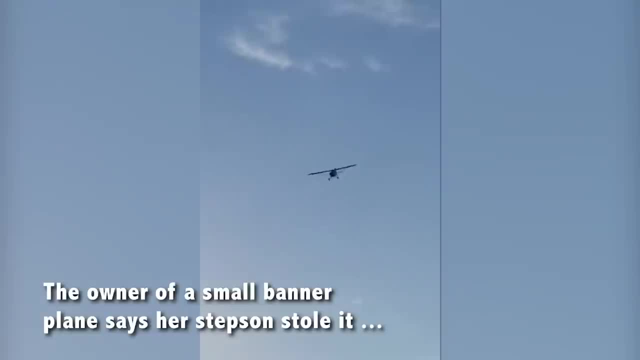 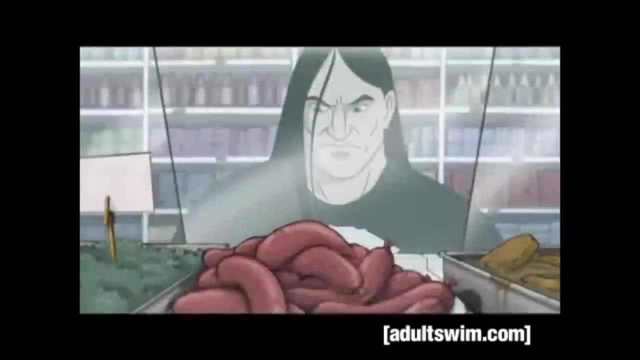 numbers and dumping or selling for scrap any traceable components, or to take the bike for a brief joyride and then dump it, the latter being less common. To decide what bikes are on the menu to be stolen, bike bandits will usually go shopping. at locations they can expect bikes to be visible and accessible. This might mean cruising neighborhoods, looking in driveways on streets, outside homes, even- in quote unquote- safe neighborhoods where people might not expect a thief and so don't take even rudimentary anti-theft precautions. 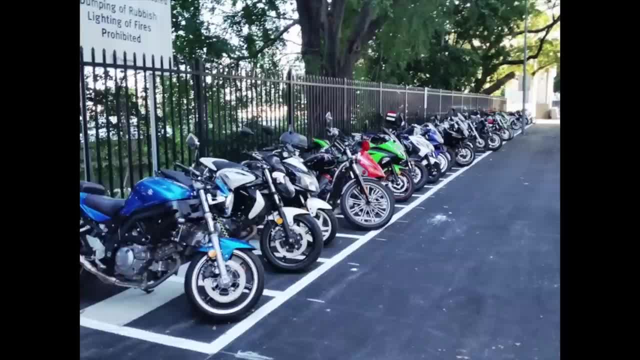 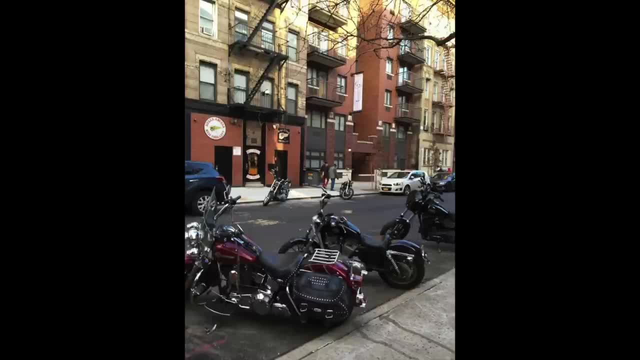 Often, potential robbers will shop at places with dense populations and unsecured parking situations, Places like apartment complexes, shopping malls, colleges or open parking lots. Once the target is determined, there are two primary ways that bikes are nabbed: The team grab and go method or, more commonly, the one man show. 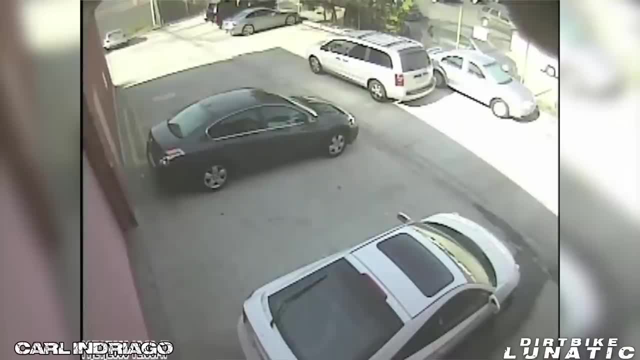 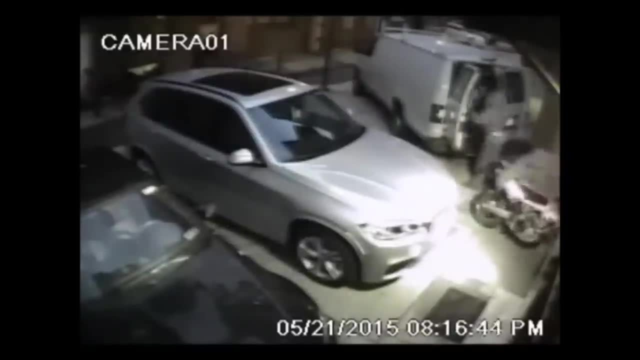 The multi-man grab and go involves multiple people driving up to a parked motorcycle and either throwing it in the back of a truck or the rear of a van and taking off. This has the advantage of being very fast, as it can take less than 15 seconds for a. 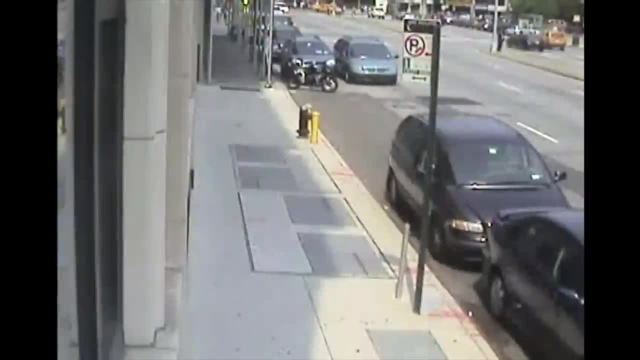 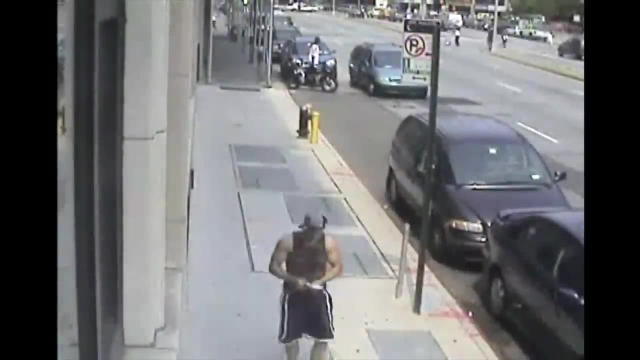 few dudes to jump out of a car and drop a bike in the back. However, it's pretty risky for thieves, as recording devices are fairly commonplace at even the worst apartment complex or parking lot, so the plate of the vehicle could be recorded and tracked down. 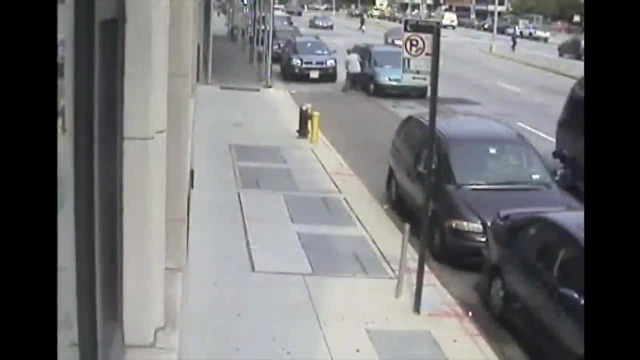 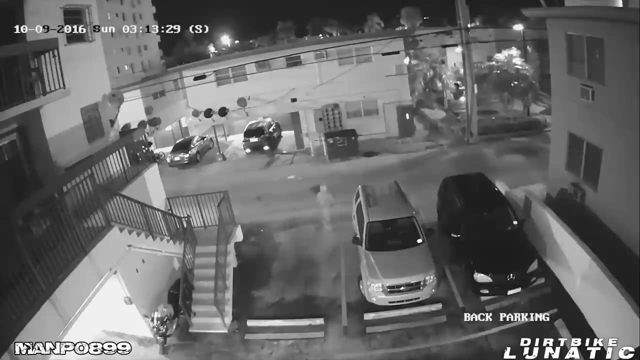 Of course they could just obscure or remove the plate during the actual heist to make it a bit harder, but make and model would still be recorded and likely fairly simple to track down. The more common theft strategy is quick and only involves one person. 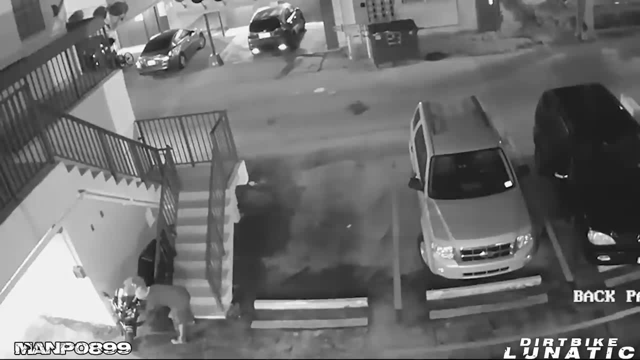 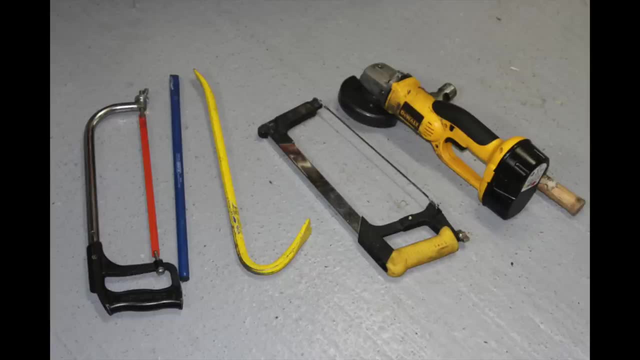 The thief walks up to the motorcycle at an opportune moment, maybe gives it a jiggle or a knock to test for anti-theft motion sensors, as well as motion lighting and other common simple security measures, Then, with just a handful of tools, either accesses the ignition wiring, maybe even 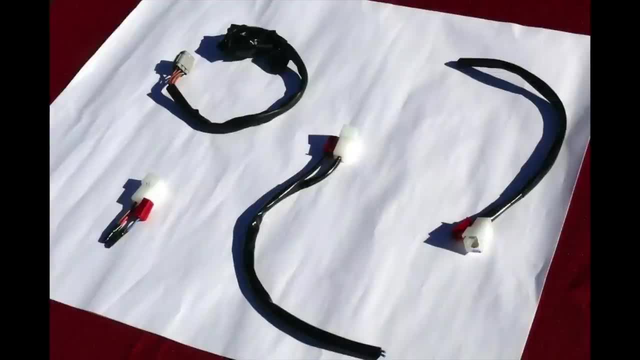 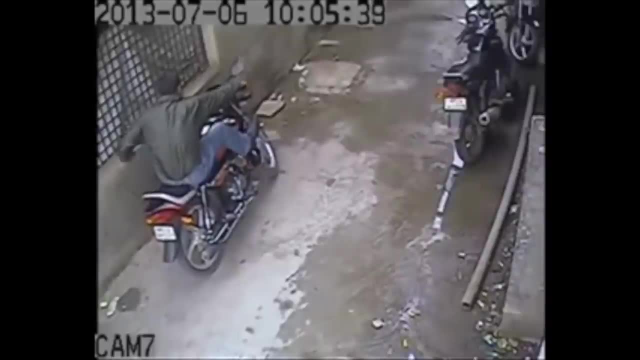 bringing their own model specific wiring harness if it's newer or harder to hotwire. model breaks the steering lock. you do use the steering lock right And rides away. For an experienced individual, this can take between 30 seconds or possibly a few minutes. 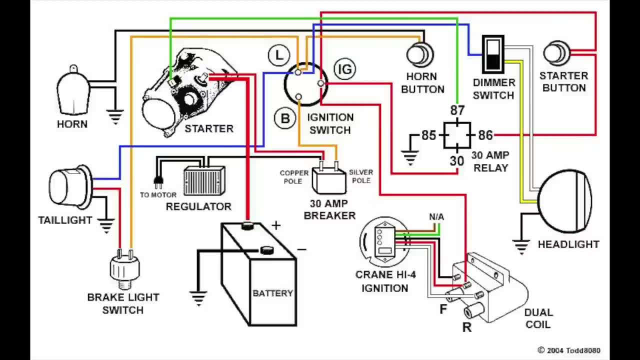 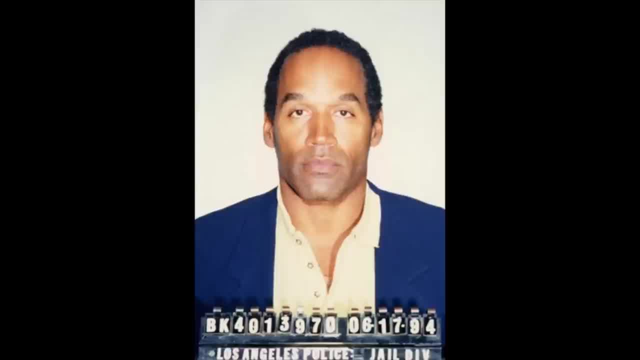 Successful thieves become very familiar with the details of each specific make and model, as well as common anti-theft measures such as lowjacks or alarms, Unless you get a clear shot of the person's face or they're seen in the act and followed. it's nearly impossible to track down a competent thief before your bike is parted out and mailed to 60 different corners of the earth. If someone does catch them in the act, risk of apprehension is low, as they can simply flee on foot and find a different score the next night. 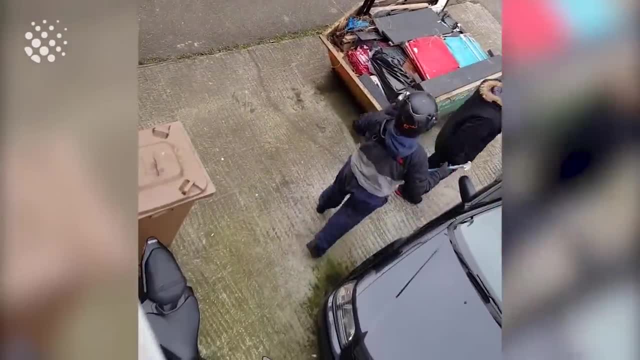 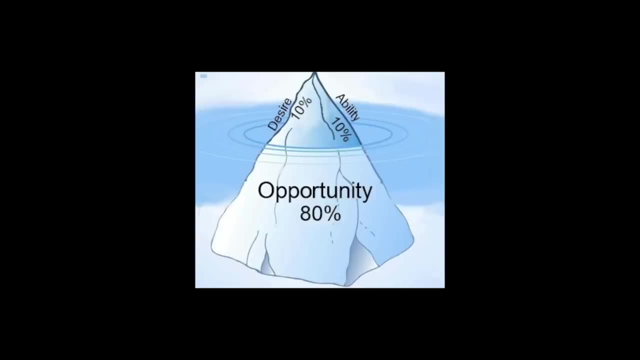 As you might expect, thieves prioritize methods of theft that are quick to execute and can be done by themselves, or maybe with a knife. It's also important to keep a safe distance from other people and a few inexpensive tools. This lines up well with the theory that motorcycle thefts are predominantly a crime of opportunity. 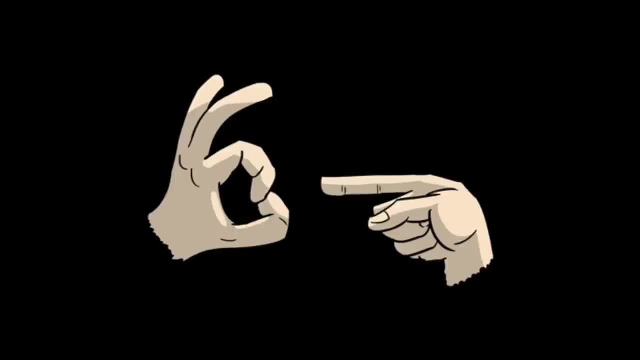 Alright, let's put this information together to work out what the best tools and strategies are to avoid theft. Anti-theft tactic one: security by obscurity If you leave your bike sitting outside all the time, especially in a high risk area, as 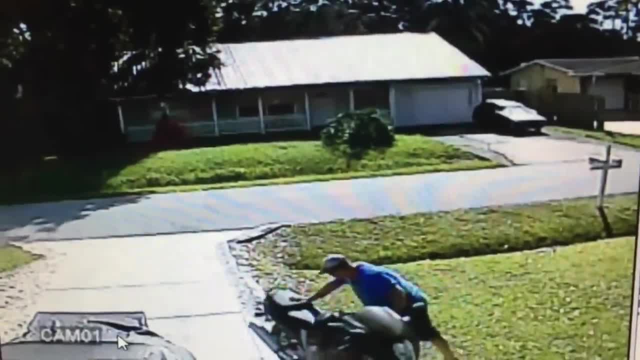 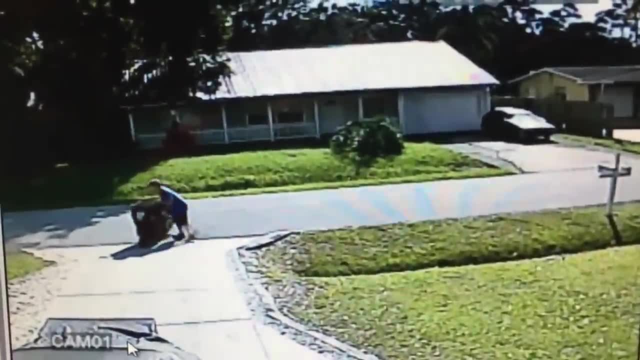 we discussed earlier. it gives plenty of opportunities for thieves to see and access your bike. So the first and, I'll argue, the most important anti-theft tactic is to reduce the visibility and accessibility of your bike to a potential thief whenever possible At your home or apartment. the best thing to keep your bike from theft is to keep it. 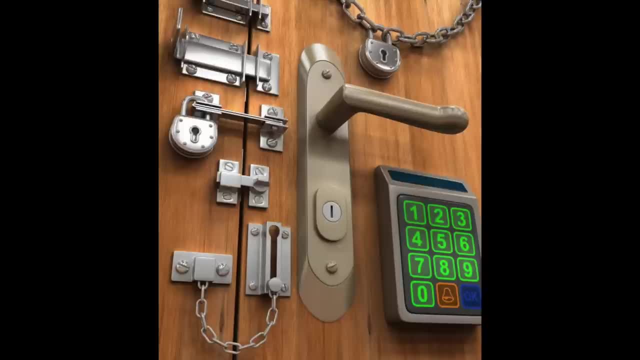 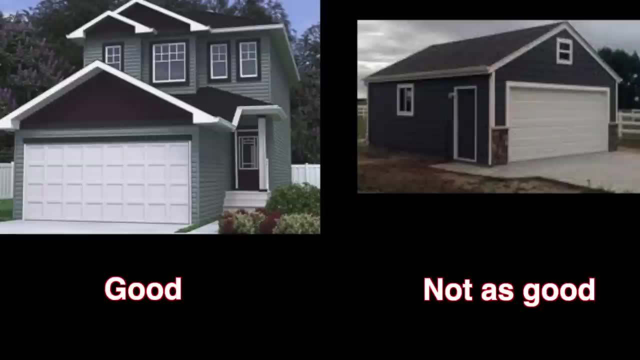 in a secured garage, somewhere that's locked up, not shared, without any windows to check the contents from the outside and connected directly to your abode, In addition to removing it from prying eyes. some thieves might consider that stealing a bike is grand theft, but once you enter someone's garage, you get into more severe. 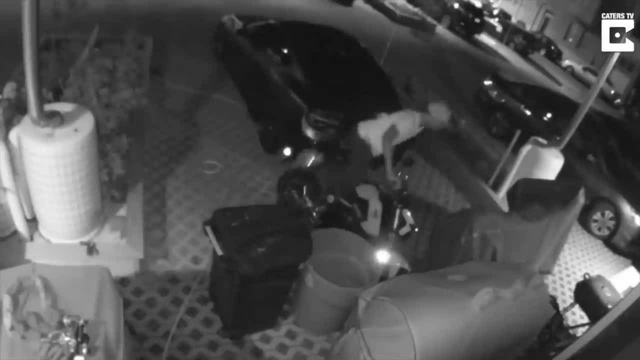 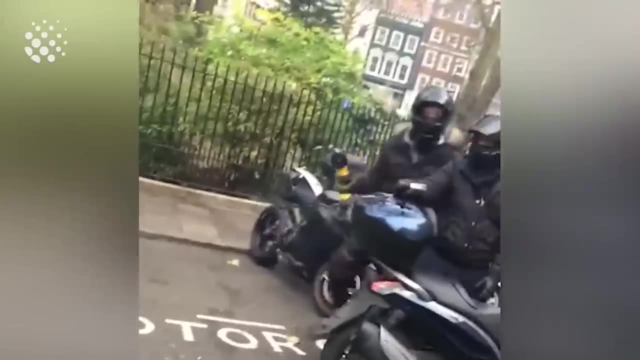 charges like trespassing, breaking and entering, and that you are far more likely to encounter the owner with a weapon than in someone's driveway. There can be a lot of challenges trying to obscure your bike in more public places like apartment complexes, as many apartments don't have secured garages or provided storage large 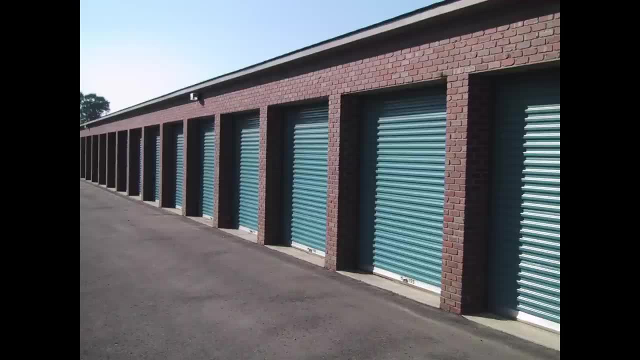 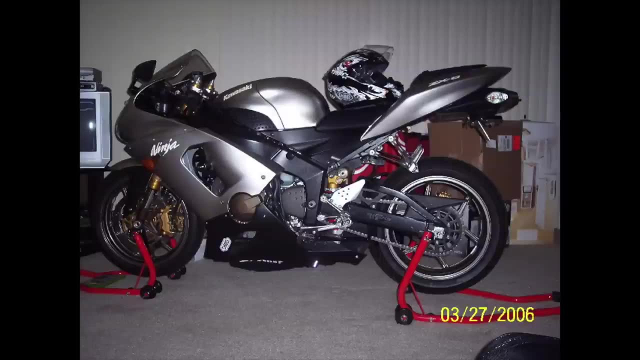 enough to fit, But your complex might have optional storage facilities somewhere on the grounds available for a moderate fee. or maybe you can get into the front door or into your living room, but be prepared to forfeit the shit out of your deposit. You could also use a cupboard to deter some thieves, but it's fairly simple to clock a style or model of a covered bike If a secured covered area isn't an option or you and your bike are away from home. that's when you have to get creative. 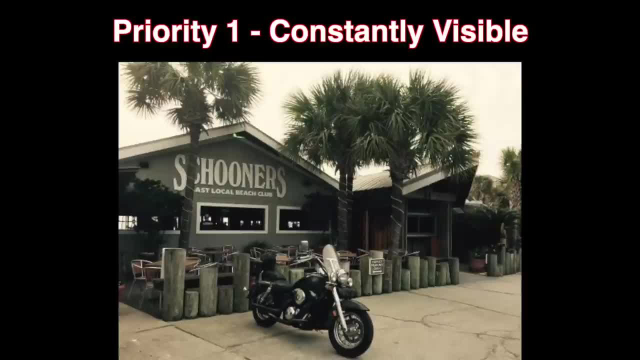 Here's how I suggest you prioritize parking and storage locations: First places where the bike is visible to you at all times while you're off of it. This is possible at places like restaurants, where there are tables and windows where you're sitting. 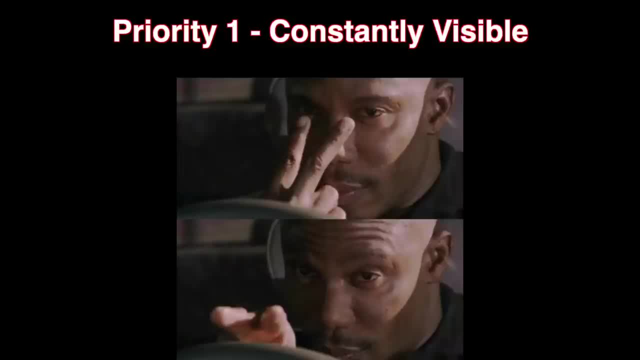 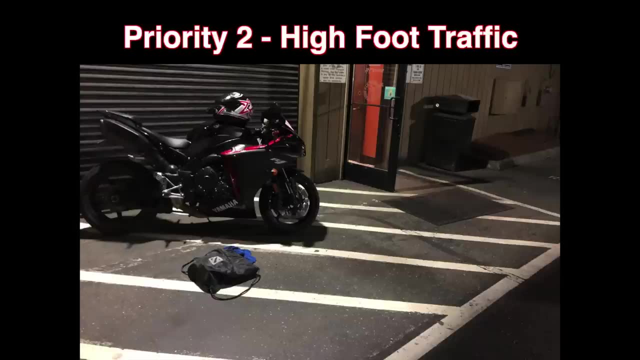 I've often parked my bike then, after being seated, moved it to ensure my bike stays in line of sight. Locations with high public foot traffic where thieves aren't likely to have time to themselves to fuck around with my bike- This is where you get into territory of pissing people off a bit by parking at the entrance. 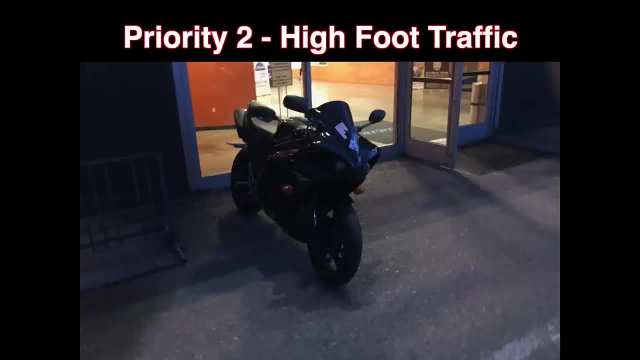 of an establishment on sidewalks or near pedestrian thoroughfares. But I prefer the mostly minor annoyance and scorn of people who don't understand the motorcycle struggle to the embarrassment and burden of getting my bike stolen, A parking garage with invisibility of- hopefully- a trustworthy lot attendant who won't let. 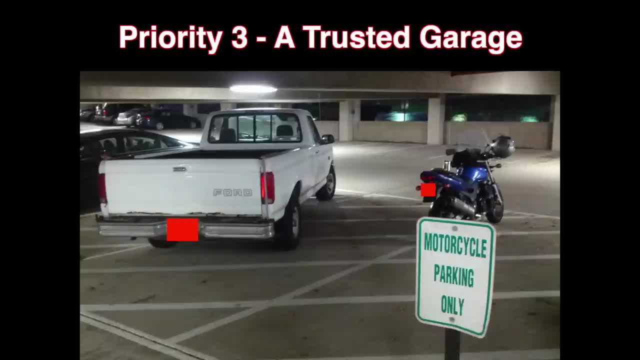 some random person start messing with your bike, As well as lights and cameras. Often this is my strategy with garages I've parked at before and trust In the nooks and crannies of a smaller, quieter garage where a thief might be less likely. 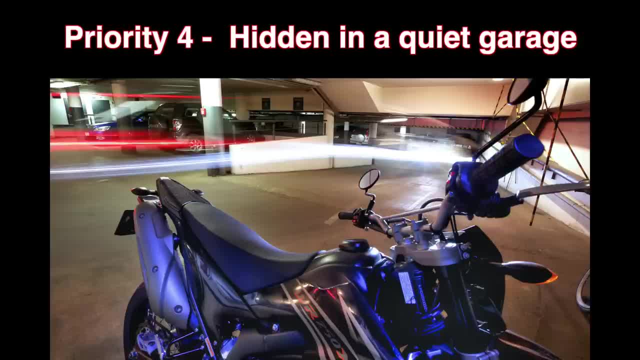 to case Now. these ideas are just how I prioritize my bike storage based on the situations I find myself in. There are an infinite number of other situations that these options don't do a great job of protecting you from, So adding some actual anti-theft protection in addition is a good idea. 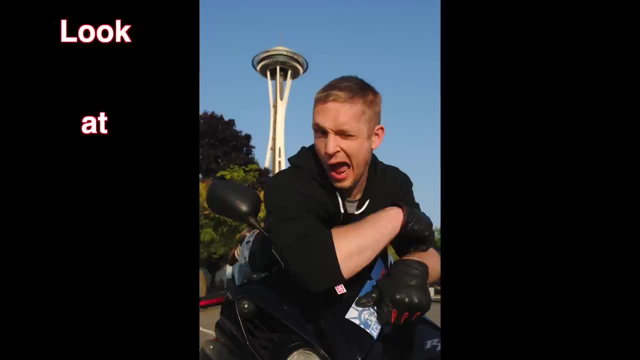 That gets us to anti-theft tactic. two: chains and locks. Video reviews and experts that talk about chains and locks seem to have a lot to say about this, So let's get into it. 1. Chains and Locks: Video reviews and experts that talk about chains and locks seem to have a lot to say. 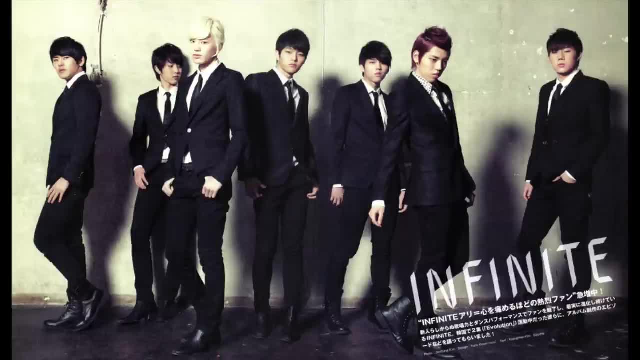 about this. 2. Chains and Locks: Video reviews and experts that talk about chains and locks seem to focus a lot on how easy or hard it is to defeat some of these simple anti-theft tools when deciding if and when to recommend them. 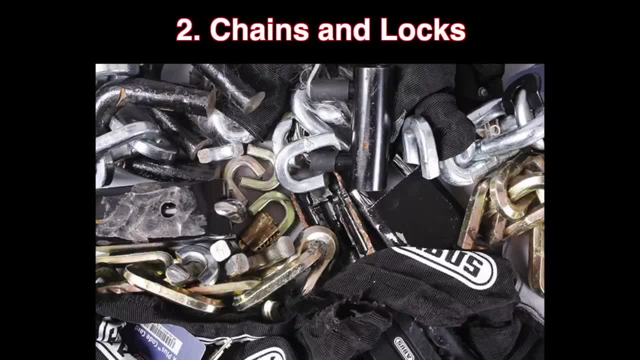 So let's get into that. 1. Chains and Locks. 2. Chains and Locks: Video reviews and experts that talk about chains and locks seem to focus a lot on how easy or hard it is to defeat some of these simple anti-theft tools. when deciding if and 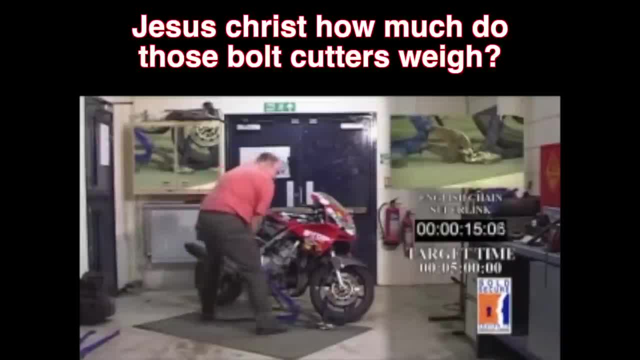 when to recommend them. The mentality that you should have when considering these mechanisms is that they are simply ways to increase the opportunity cost of stealing your bike. By requiring thieves to carry additional tools and increasing the estimated time to steal your motorcycle, you make it more or less easy to do so. 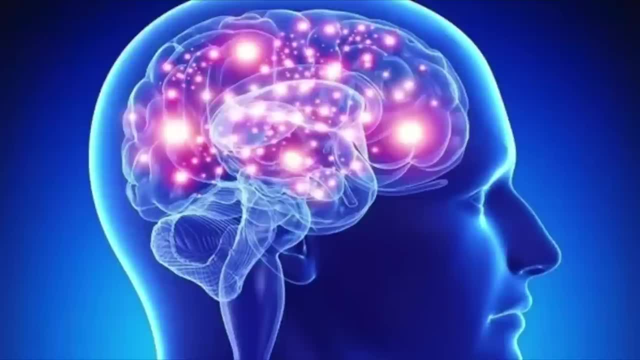 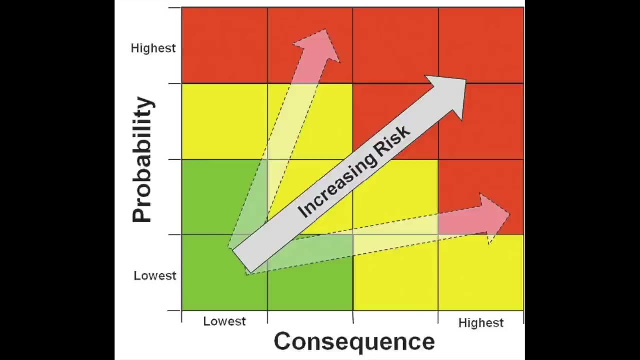 3. Chains and Locks them. The mentality that you should have when considering these mechanisms is that they are simply ways to increase the opportunity cost of stealing your bike. By requiring thieves to carry additional tools and increasing the estimated time to steal your motorcycle, you make it more likely. 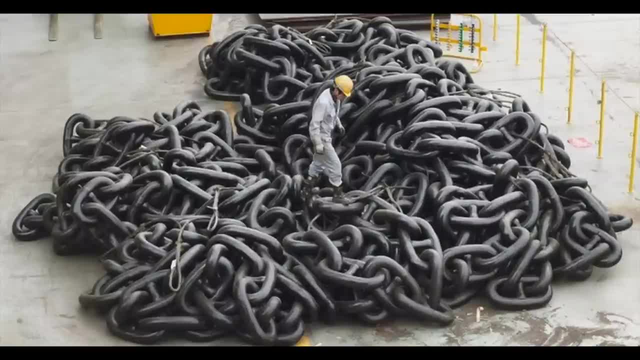 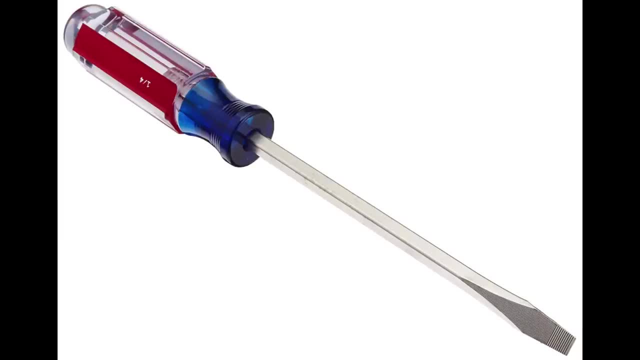 a potential thief will move on to a simpler target. You don't need the biggest, baddest chain or lock to get the benefits of dissuading a would-be thief. Just something that can't be defeated quickly with the most common tools: Hammers, screwdrivers and bolt cutters. Where 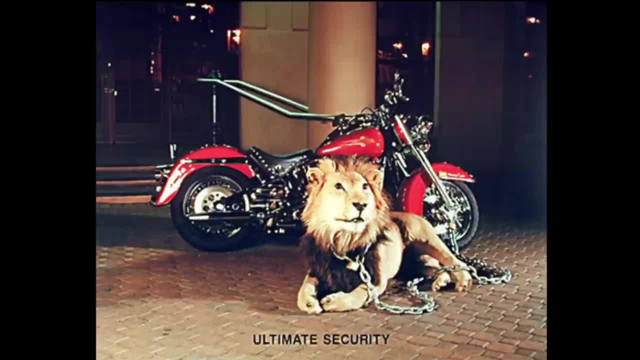 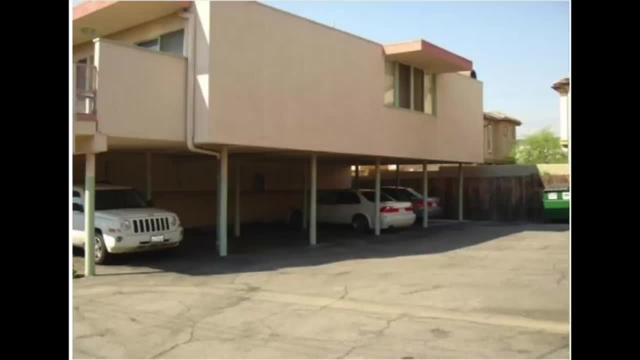 you might want to invest in heavier locking mechanisms is places where your bike has to be in riskier areas for long periods of time, Like if you work at a shopping mall for eight-hour shifts or have to leave your bike in the carport of your apartment. Getting a lock that requires 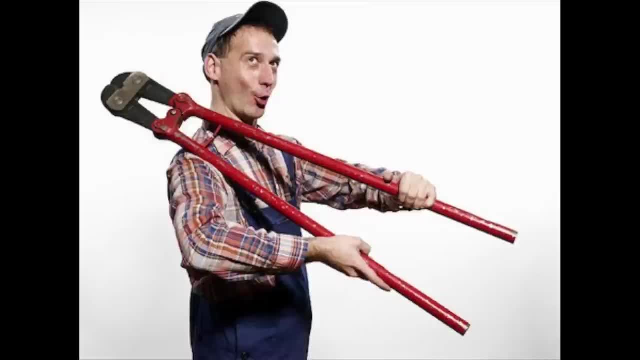 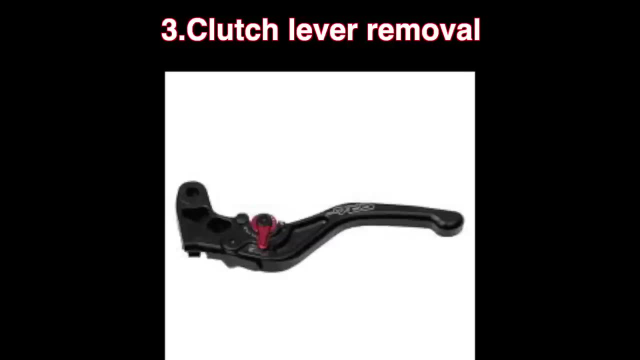 heavier tools than a single thief will want to carry can do a yeoman's job of dissuading all but the most determined and prepared thieves, as most aren't going to carry jaws-of-life-grade bolt cutters. Anti-theft tactic, three Clutch lever removal- One anti-theft tool. that is basically. 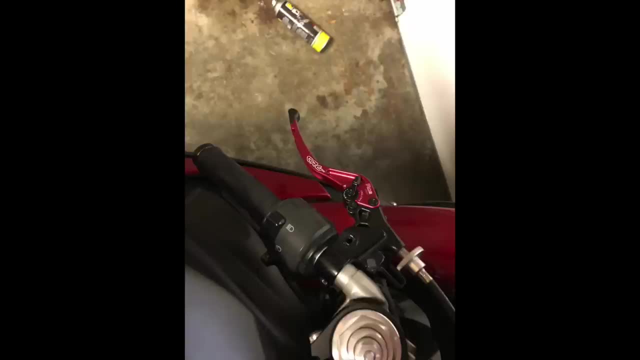 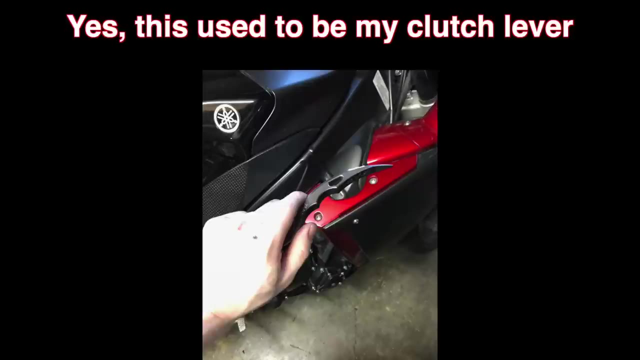 free but somewhat more extreme step you could take to dissuade a thief is to keep a flathead or whatever tool with you and remove your clutch lever when you park your bike. This is something I might resort to if I knew I had to park in a very bad area and I didn't have a chain. 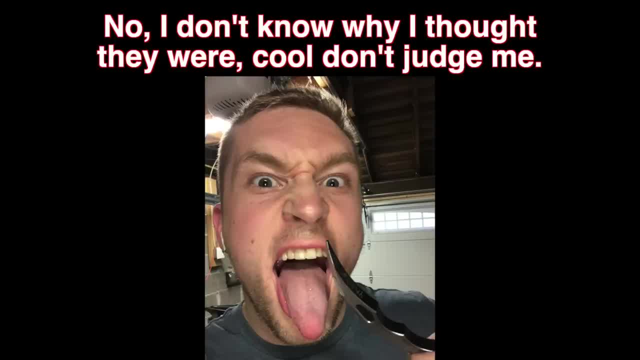 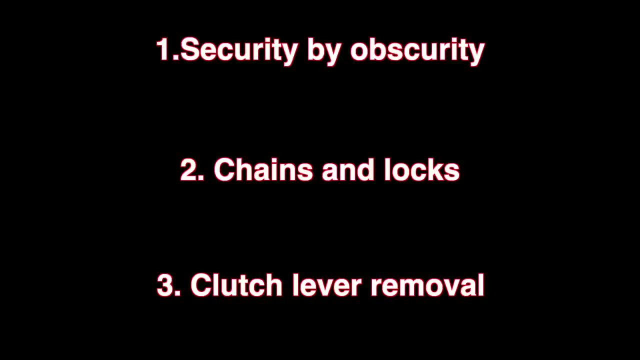 or a lock with me. This is, of course, much less effective if you park in a bad place seven days a week, as eventually a thief might just bring their own lever. These three tactics are pretty much all I focus on for my theft prevention, as they're simple, effective. 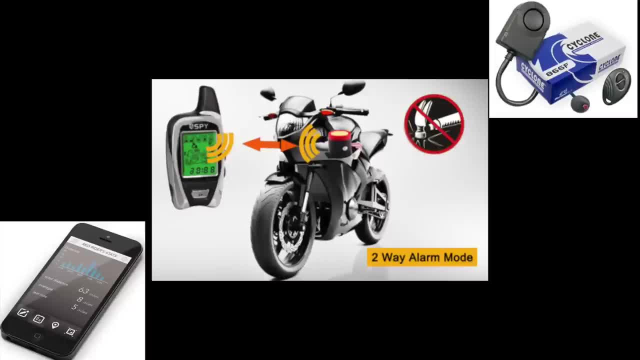 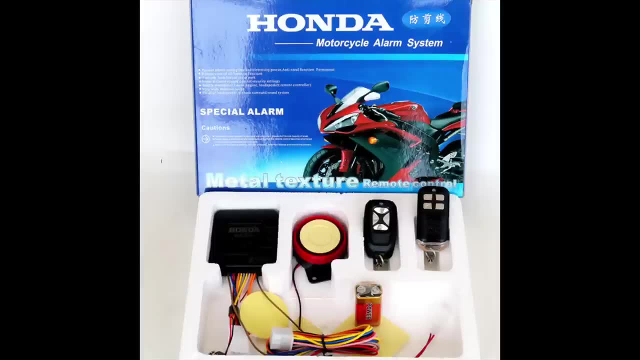 and low-cost or free. Of course I've left out a lot of other anti-theft options. Let's cover those too: Alarms and lowjacks. You're probably curious why I don't necessarily recommend electronic anti-theft systems like alarms and lowjacks, especially since I've had multiple 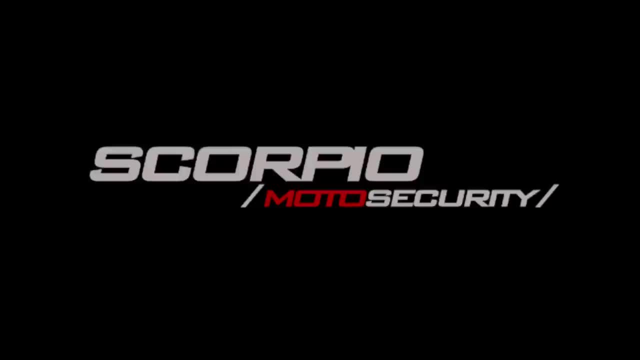 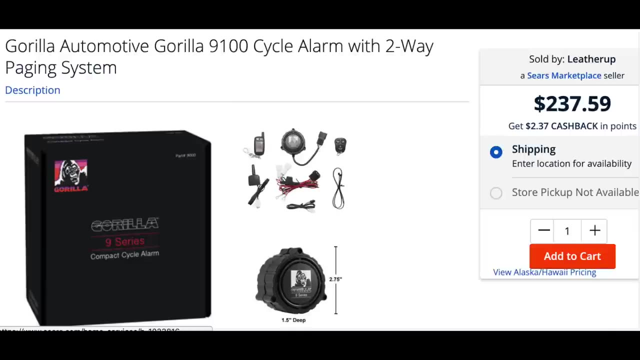 bikes stolen. I did use a Scorpion full alarm system for a spell, but I found there are a few nuances that make these devices sometimes a hassle or less effective than they seem. Comprehensive alarm systems are prohibitively expensive for many people. Something that has a combination. of useful features like motion sensors, GPS tracking, app connections, mobile notifications, remote disable, etc. tend to run in the hundreds of dollars. That's not including installation. if you aren't a gearhead or don't want to take the time to do it yourself and a poorly 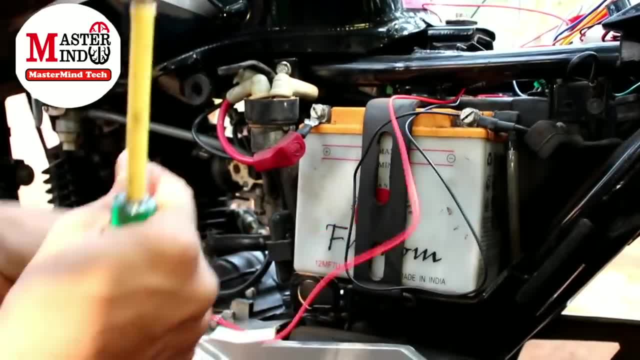 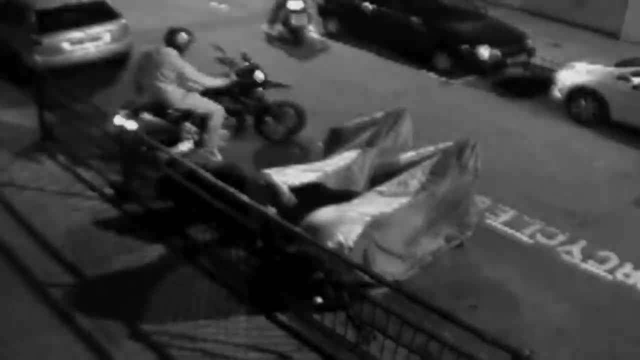 installed alarm system that can easily be disabled reduces its effectiveness significantly. They also don't keep thieves from attempting to steal your bike in the first place, the way something obviously visible like a lock or a chain do. Location devices like lowjacks and GPSs are also found to be a bit troublesome. Some of these systems require a monthly or 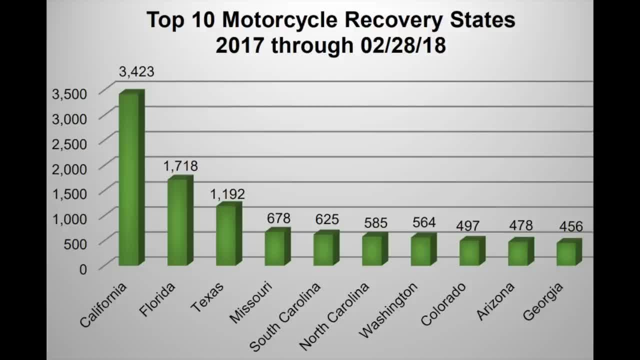 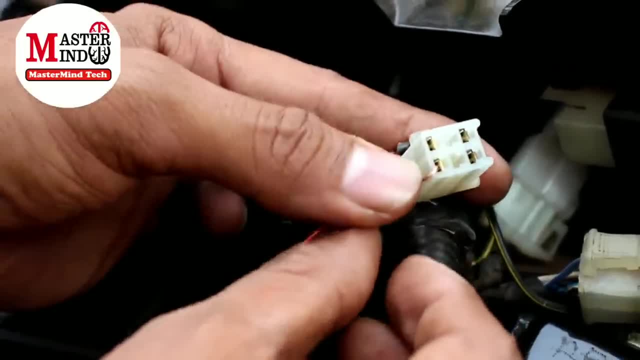 yearly fee on top of the upfront cost, which isn't awesome. They also only give you the hope of recovery after it's stolen, opposed to preventing it in the first place. A competent thief knows to check for these devices, and a poor installation can allow a device to. 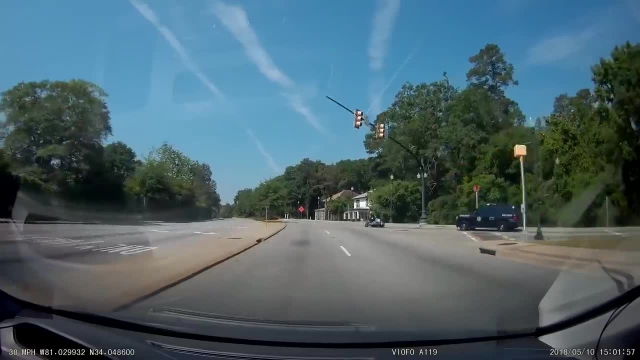 be found fairly quickly before you even realize it's gone. Unless you're able to immediately start tracking your bike after it's stolen, or your bike's been stolen for a long time, or your bike's grabbed by a complete amateur, it might not even do a great job of its intended. 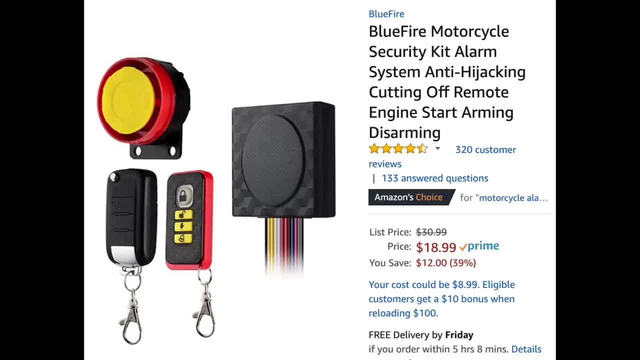 purpose. Now there are simple electronic anti-theft tools that are very inexpensive, that have motion-activated alarms, and these can dissuade a thief that's unprepared for it. But if you or nobody else responds to the alarm, then it might only be a temporary. 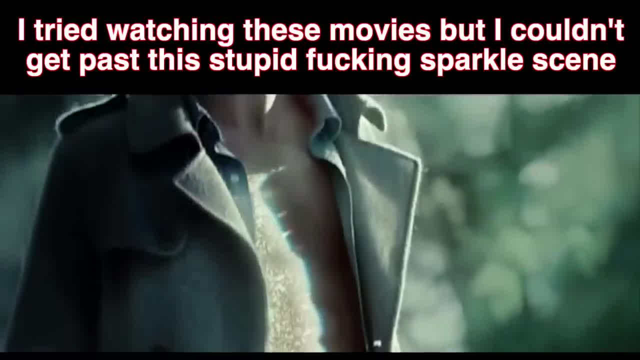 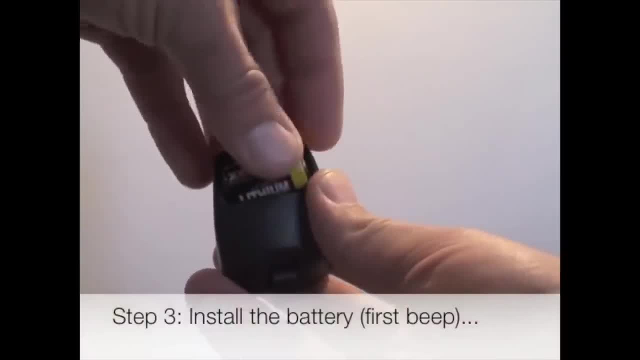 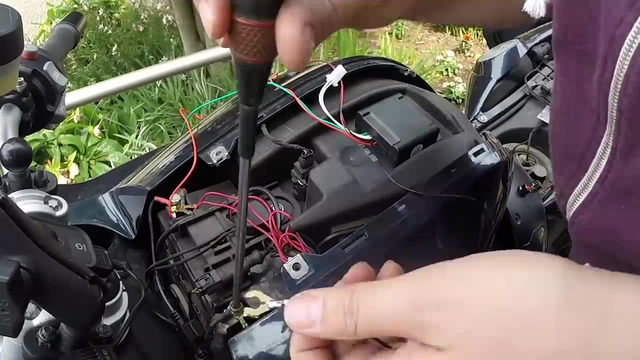 deterrent. There's another problematic aspect of these additional electronic components: vampire power drops. For these alarm systems to function, they require power. Some use their own power source in the form of a battery pack. you have to keep purchasing batteries for and making sure it's running. Others are connected to the battery directly, Depending. 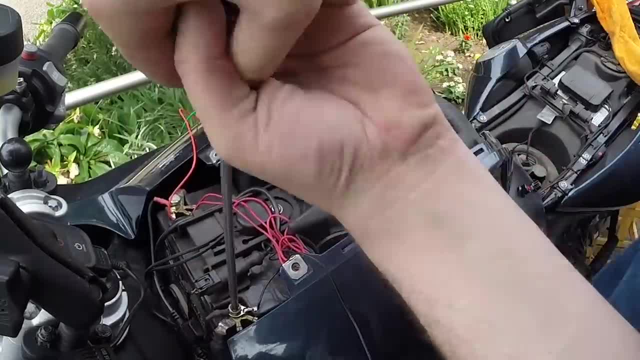 on the product and its features. you could find that having your bike off of a tender for even a few days could create a situation where there isn't enough power in your battery to start the bike. Using a tender also relies on having a place you can safely connect your 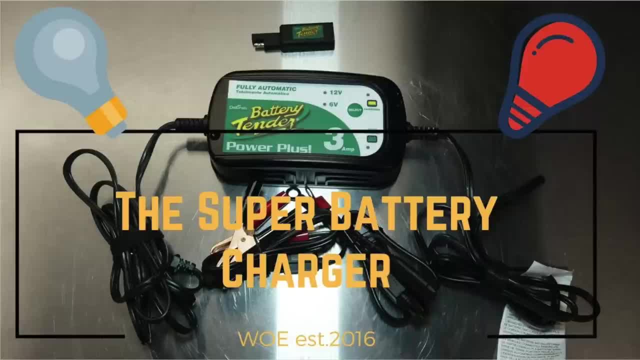 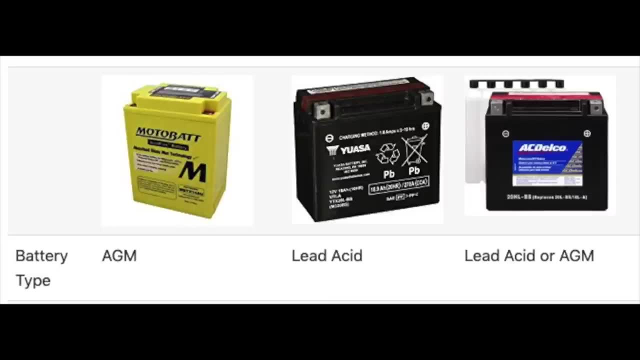 bike to power and have your battery accessible without providing access to ne'er-do-wells. On top of all, this long-term vampire draw can wear batteries much faster than normal, leading you to needing to replace your battery more often or using batteries that are more. 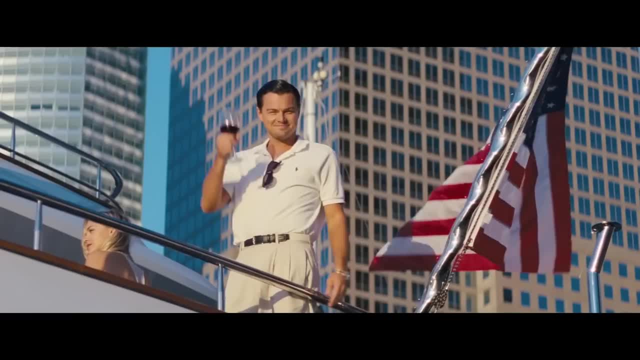 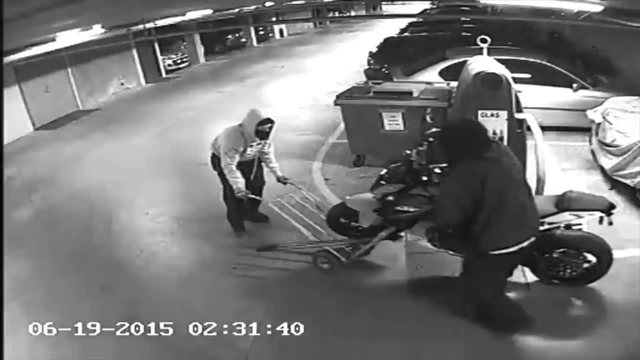 expensive to improve reliability. With all that said, if cost isn't a problem for you or if you know your bike has a significant likelihood of being stolen- for example, if it's less than 3 years old in good condition and you have to leave it in bad places for. 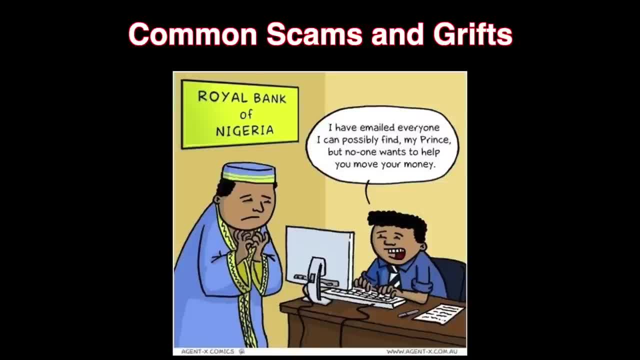 long periods of time, then one of these systems might be the right choice for you. I also want to bring attention to some common grifts. people might pull on you in order to steal your bike. At some point you'll probably want to sell your motorcycle and Craigslist 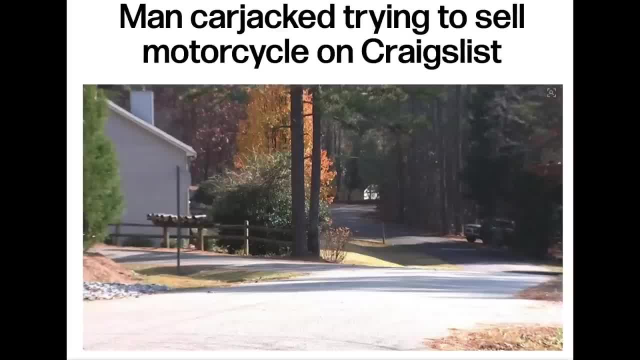 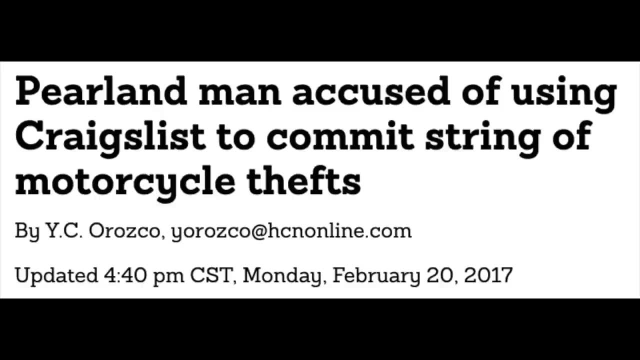 might be a place you want to use to advertise it. Whenever showing the motorcycle to someone, take it to a safe, open location away from your home. On the off chance a potential buyer is actually just looking to get an idea of where you live and security measures your 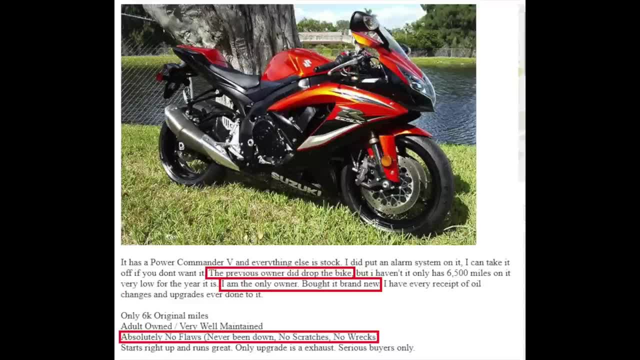 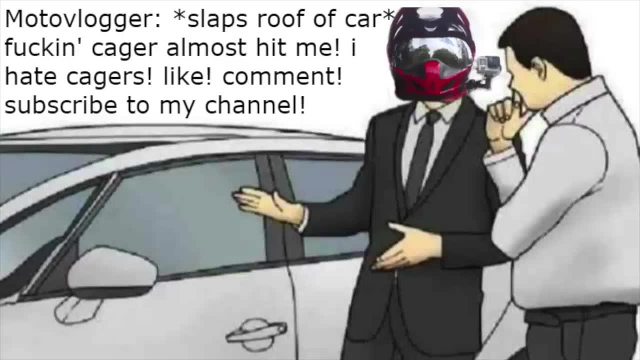 bike may have. Don't buy a bike from a private seller. Don't give them any more information about you or where you live than is needed, even if the bike is a steaming good deal- Shady shops. If you buy a bike from a shop, you have to give them lots of information. The 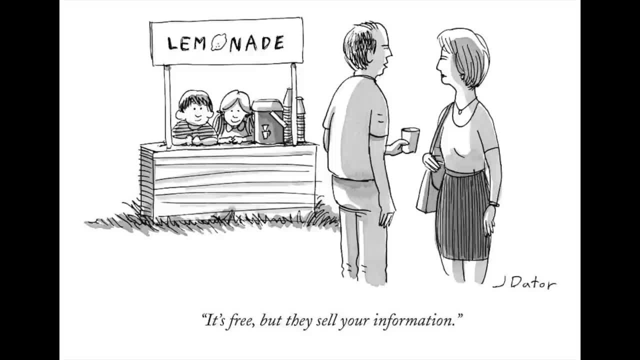 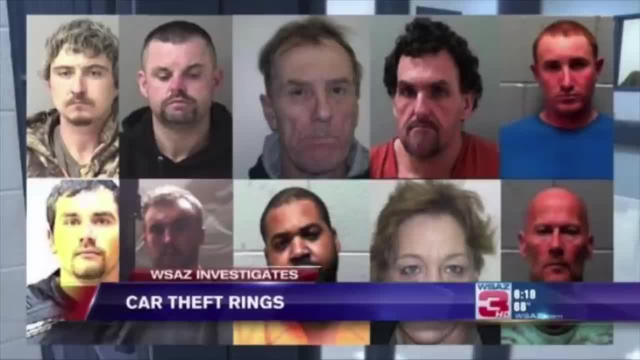 sad part is there are a lot of people that have access to all of that information and know all the details about you and your brand new bike. You probably can't know for sure if a place you're buying from has someone scoping out marks for them. but don't wait. 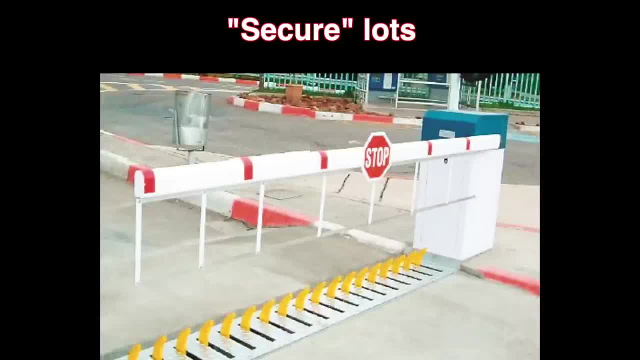 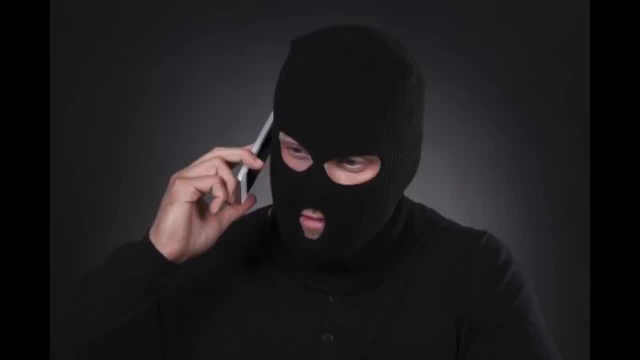 to put any theft measures in place with any new bike. Secure quote, unquote lots, Like I mentioned before about garages, don't treat garages or fenced-in parking lots as if they're Fort Knox. Employees and attendants can easily phone a friend and conveniently walk away. 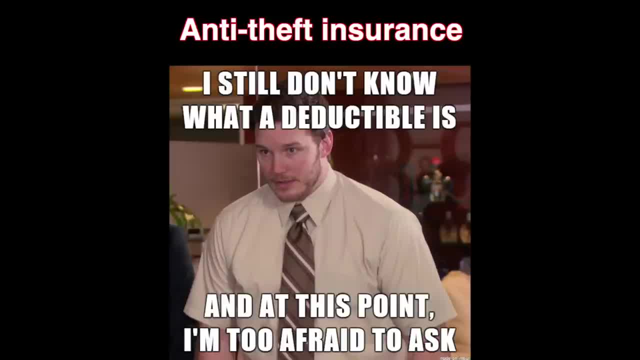 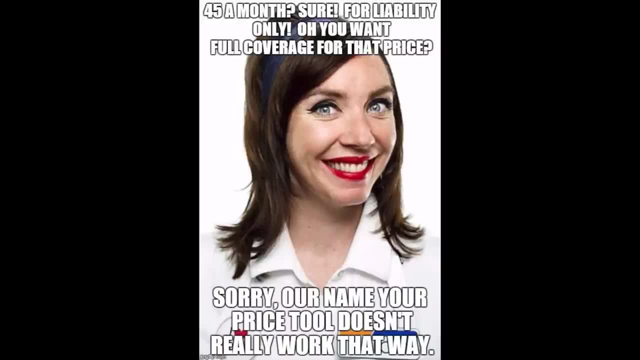 from a post or location at the right opportunity. Finally, let's talk insurance, Because after all that theft talk, you're probably feeling a bit paranoid and are probably calling your insurance company right now to upgrade your liability to full coverage- The mentality that the only real anti-theft protection is. 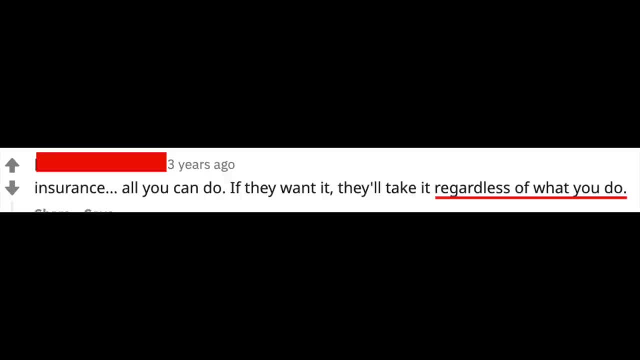 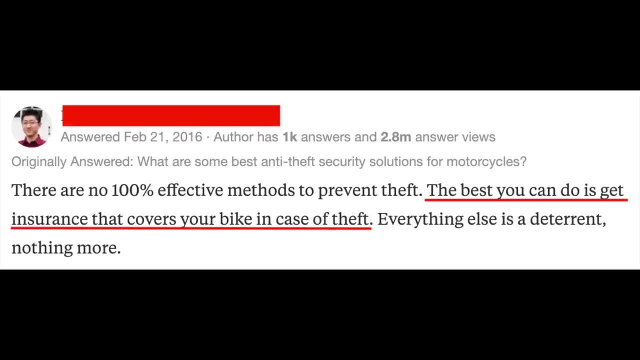 insurance is pretty common and it's probably not a bad perspective to have, assuming that it doesn't lull you into a false sense of ease where you don't take anti-theft steps like I described here, But if your bike's stolen it's still going to be a major hassle. 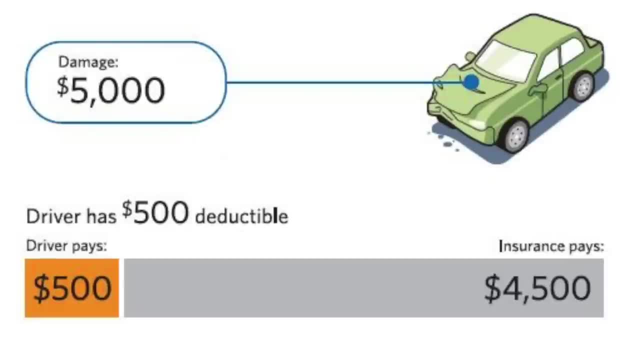 for you and likely cost you a fair amount of money. with insurance, First you have to pay your deductible, which many of us opt for- the higher amounts to reduce cost, putting you likely in the $500-$1,000 range up front if your bike gets lifted. Second, 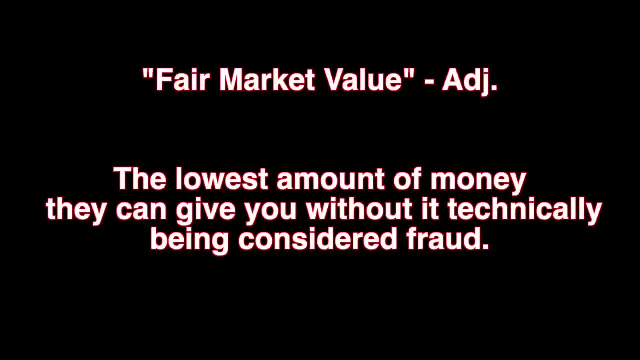 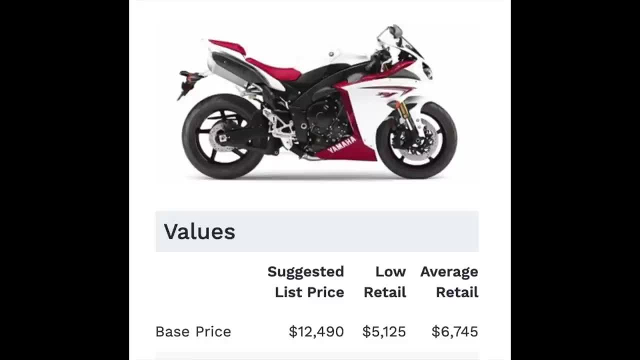 the way most insurance companies decide how much money to give you is based on this nebulous term of fair market value. This usually means they'll check private sellers and shops for your make and model to see what your bike is going for today and offer you a sort of lowball average of those prices. If you had any accessories you want to be reimbursed for, you likely need to prove you bought them and that they were on the bike. Some insurance policies require covered accessories are professionally installed. so even basic stuff like clutch levers you installed yourself won't be covered, Even if you jump through. all those hoops, they'll likely still only cover up a specific dollar amount of add-ons, usually about $1,000.. After they tell you the disappointing amount of money they're going to pay you for your beloved bike, you get to play the waiting game while they sit. 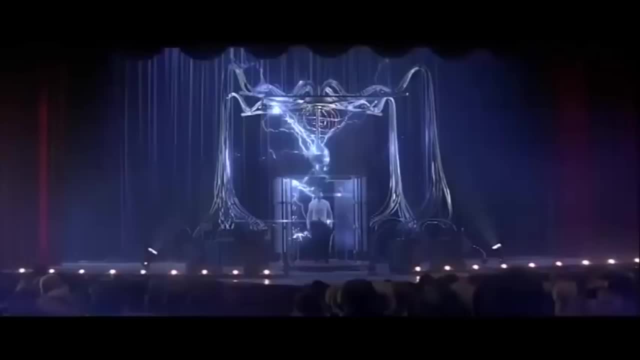 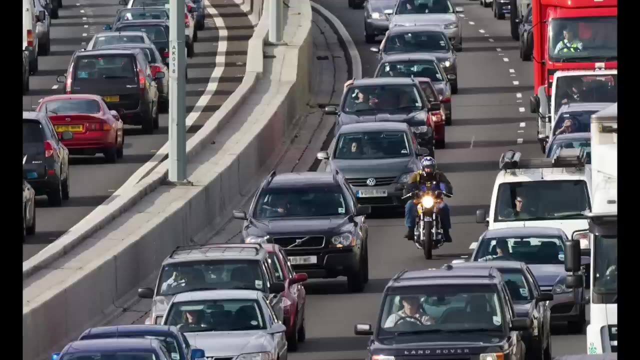 on your money for a month, hoping your bike magically shows up somewhere in pristine condition. Yes, because many insurance companies consider a motorcycle a recreational vehicle and don't consider or care that a motorcycle might be your primary means of transportation. they'll make you jump through that hoop too. Finally, after the dust has settled on your claim, 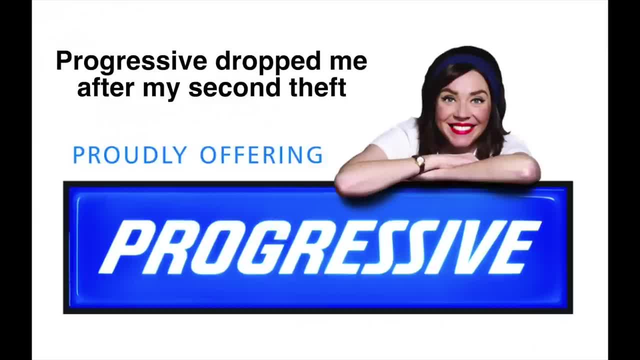 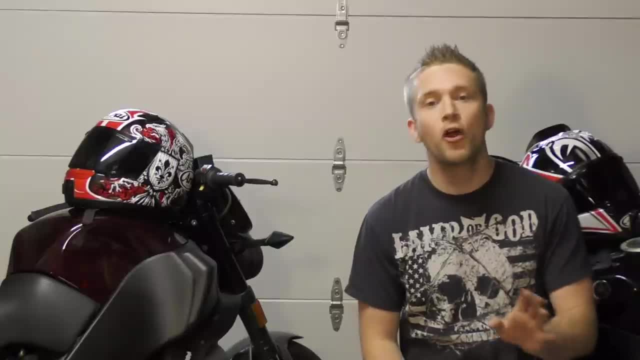 your insurance company might drop you if you have tickets or other things they consider increased risks. Thanks, Progressive. So yeah, insurance that covers theft is an option, but Joe will help you if you have to actually use it. Look, I hope you never have to go through having your motorcycle stolen. I eventually. got to the point with my bike where I bought two huge chains and put one at my apartment complex tied to a giant metal pole outside my bedroom window and the other at my work tied to another giant metal pole at the front of my building. It was super effective. Hopefully all this theft talk doesn't give you too much anxiety. 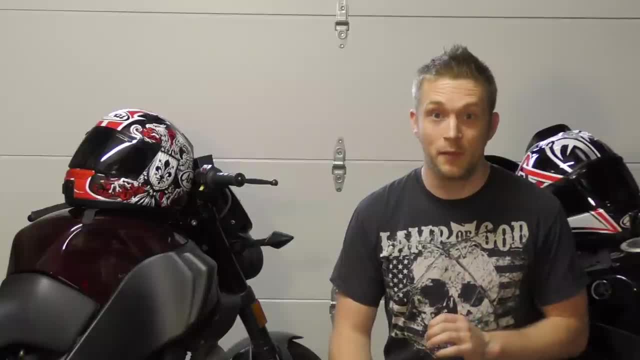 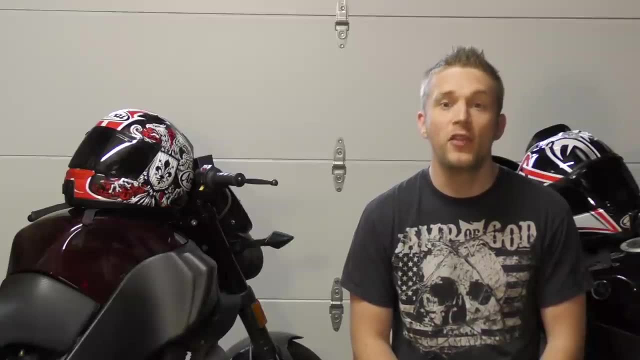 but if your motorcycle gets stolen, you'll definitely have a lot of anxiety about your next bike. Ugh, that's kind of a downer. Maybe I should insert like a fart noise or something here to lighten the mood. Nailed it In separate news, we did it. I'm officially on my way. 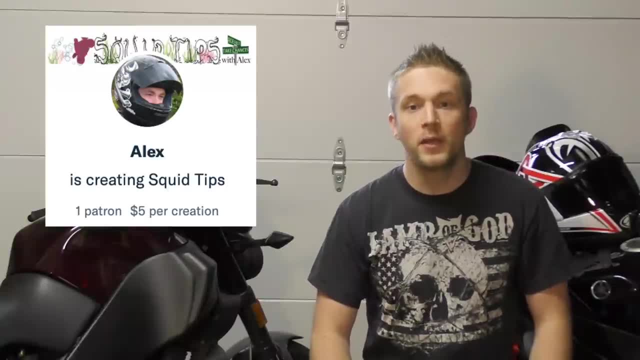 to recoup the frankly dumb amount of money I've spent creating these videos, because we now have a Patreon subscriber. Thanks, PatrickDK. I bought myself five dollars worth of Levee's and I'm going to give it to you. Thanks, PatrickDK, I bought myself five dollars worth of Levee's. 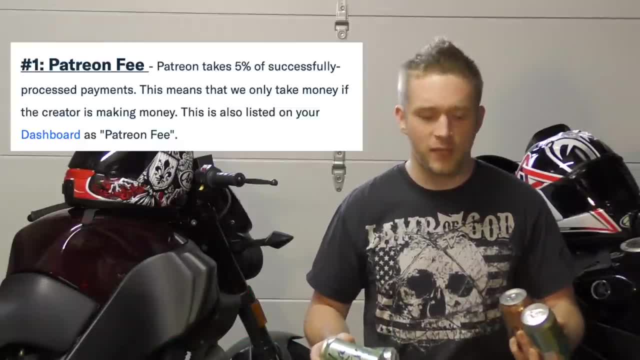 and I'm going to give it to you. Thanks, PatrickDK. I bought myself five dollars worth of Levee's- you know, Lecroy- to celebrate, Although Patreon takes a cut. so I think I'm 20 cents. 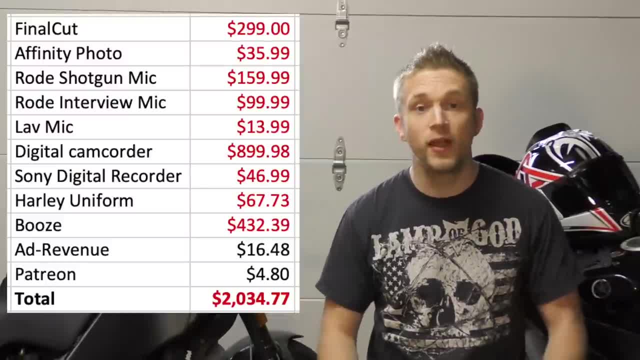 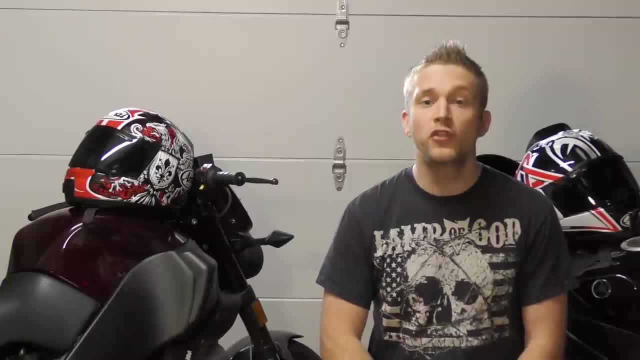 in the hole on these. Of course, since we're still in the red here, I had to take another sponsorship. Cartoon Network's Adult Swim is now looking to push a new family-friendly image, so they sponsored today's video and asked me to show you some clips of a wonderful 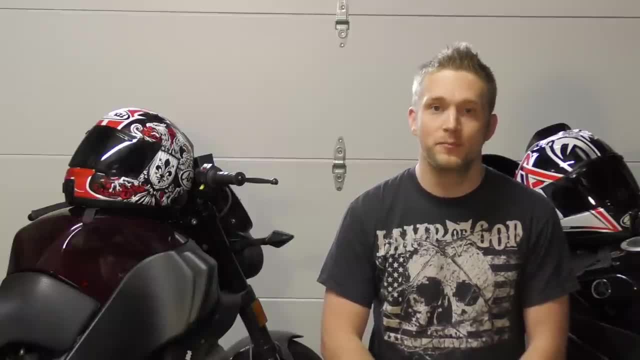 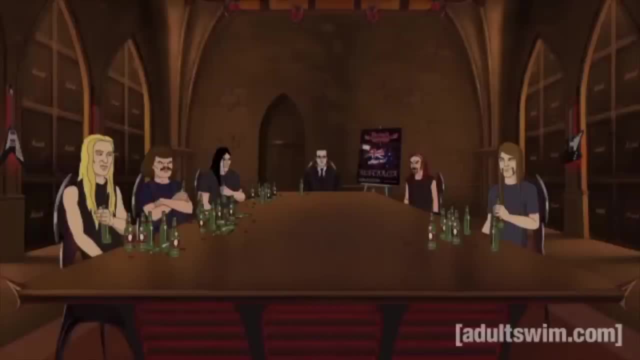 show that's now been off the air for about five years: Metalocalypse. Hey, my father's dead and I'm totally fine. What am I supposed to do without balls? It's my whole life. You could eat an apple. You could always eat an apple Instead of drinking. 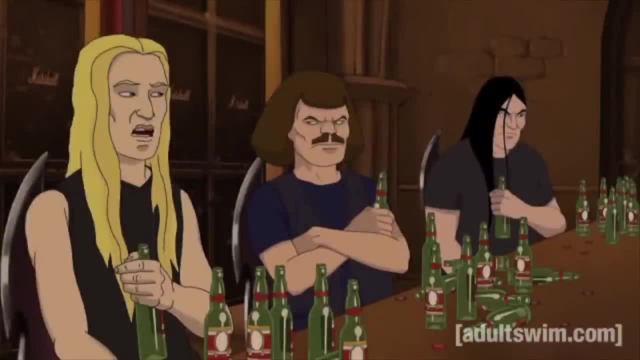 You can try, instead of doing drugs, jacking off while you choked yourselves with a leather belt around your throat close to the point of death. Yeah, that's a natural high. Yeah, that's good, clean fun. I do it every morning. 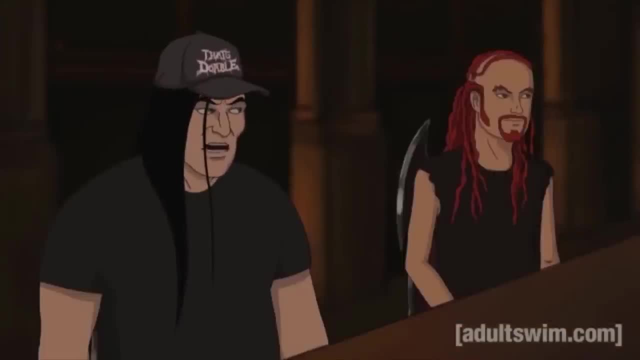 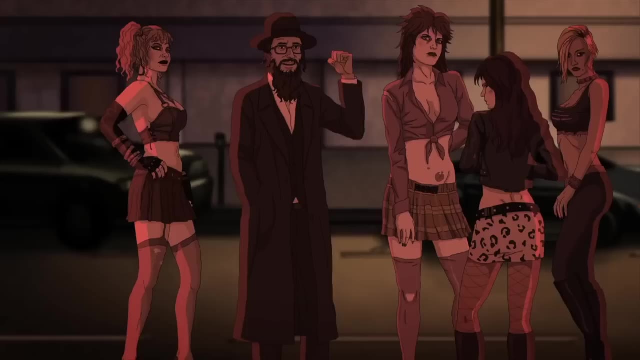 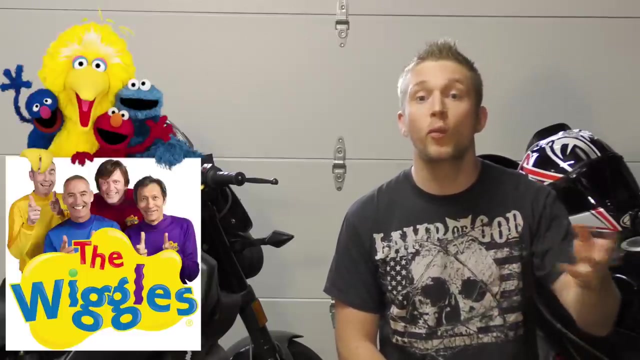 They're calling you racist. We're not racist. We don't give a f*** what color our fans are, because we don't give a f*** about our fans. Yeah, so just go ahead and show that to your kids. in between Sesame Street and the Wiggles episodes: 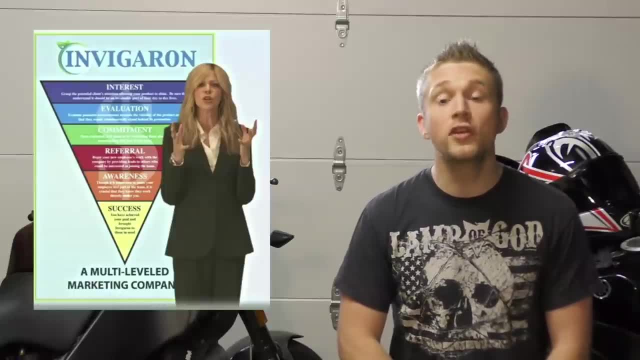 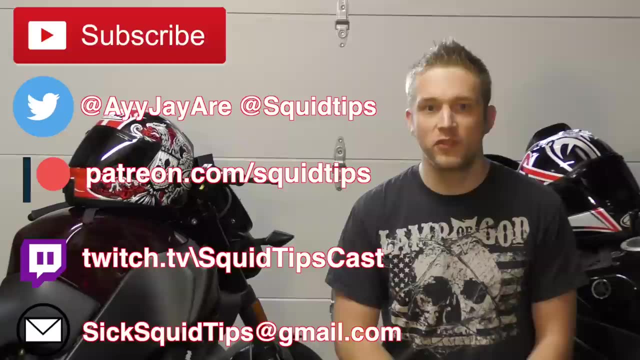 If you'd like to help me not have to go back to multi-level marketing schemes, you can help me out on Patreon. Of course, you can also subscribe, follow me on Twitter or Twitch for more of this garbage. I know I've been a bad streamy boy this summer. I'm sorry, It's been busy. I'll get back to it in about a month. 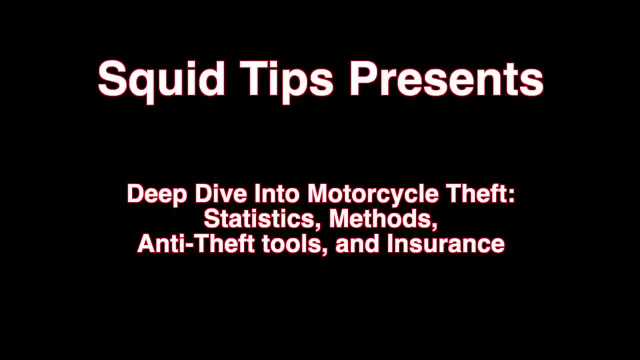 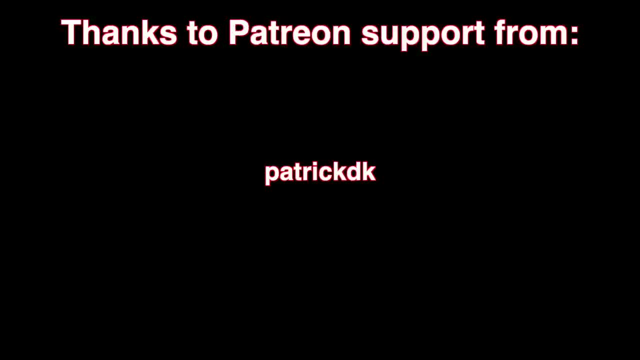 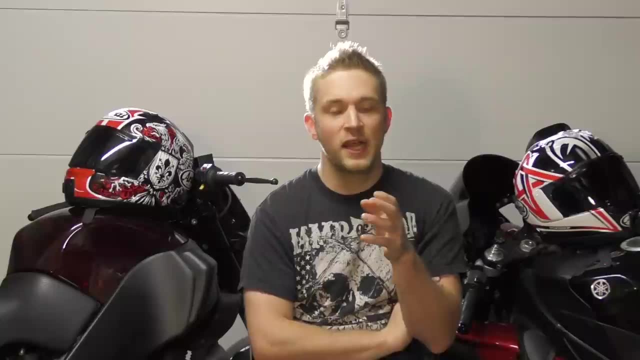 Write fast and take chances. The story of my motorcycles getting stolen are actually connected to each other and it's pretty f***ing ridiculous. I was living in Vancouver, Washington, and me and my girlfriend at the time went over to Portland, Oregon, to take some photos because we were feeling creative. 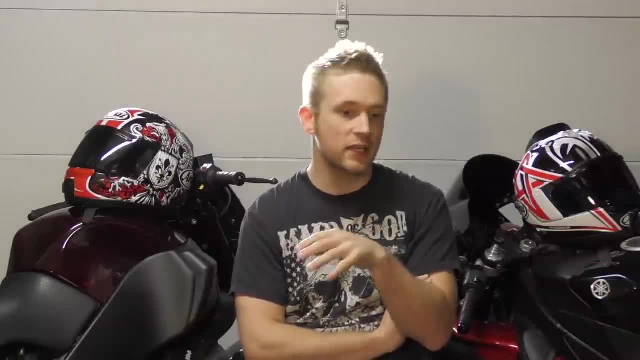 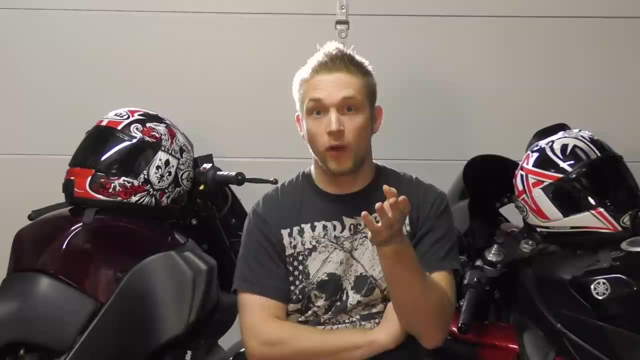 We go down to the waterfront, We go down to the Lamont River, We're taking photos, having a great time. We're probably gone, all in all, probably three hours. I drive my 2006 R1 downtown pretty close to Pioneer Square, if you're familiar with that, and leave it there with helmets attached. 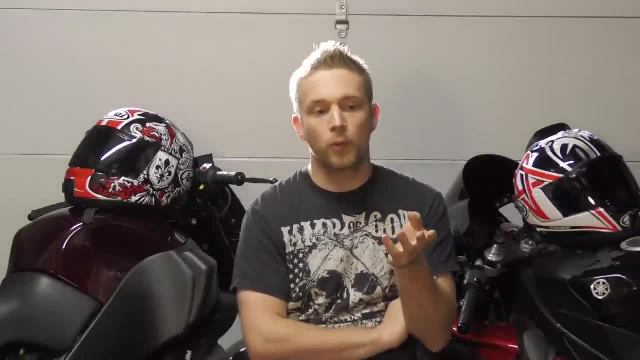 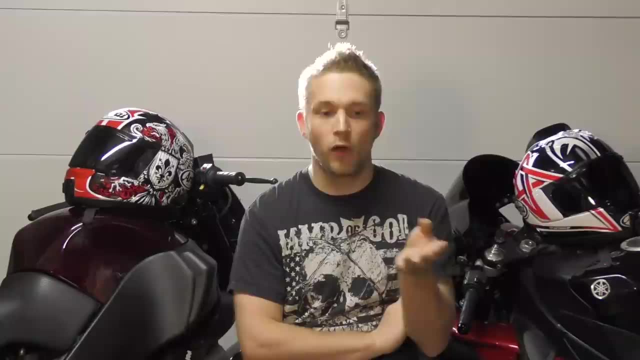 Yeah, it was pretty dumb in retrospect. All in all, we're probably away from the bike for three hours. I mean it was daytime and I had never had a bike stolen, so I wasn't even thinking about theft. Of course we come back and it's like I'm pretty sure I parked right here. 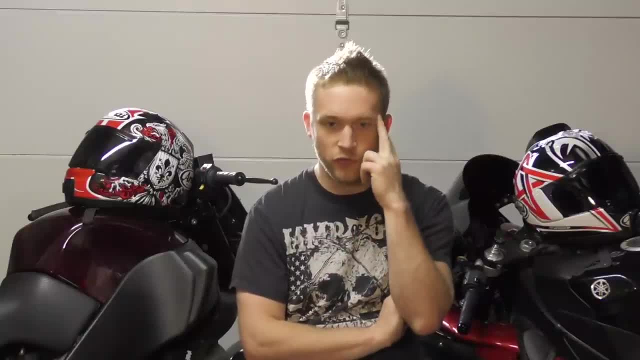 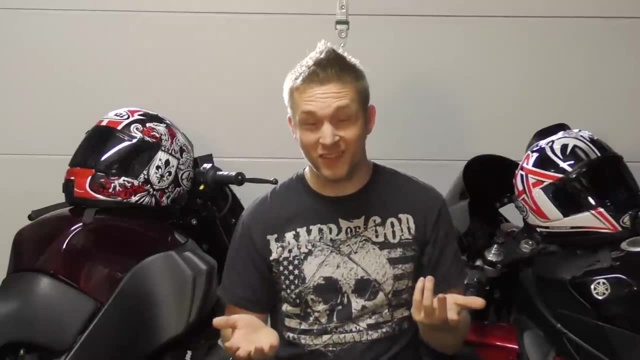 I must not have right. Then your mind goes to: oh, my bike must have been towed. maybe We go look around to see if any of the businesses maybe would have towed us. but I think it's a Sunday and they're all closed down. 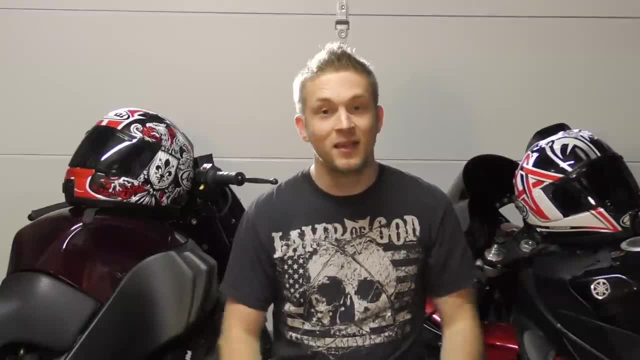 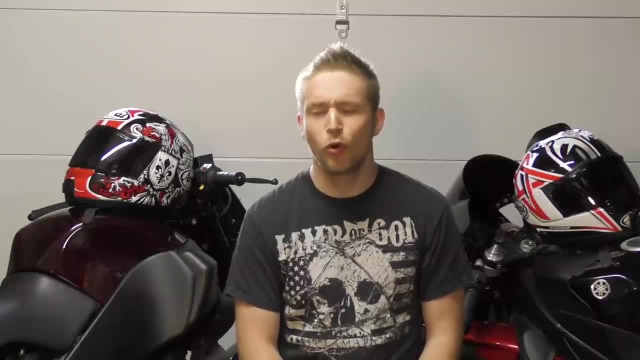 So it finally comes. It connects that, hey, my bike must have been stolen. So the police come and I file a police report and the police basically say, yeah, we're more or less never going to find this bike. just so you know. 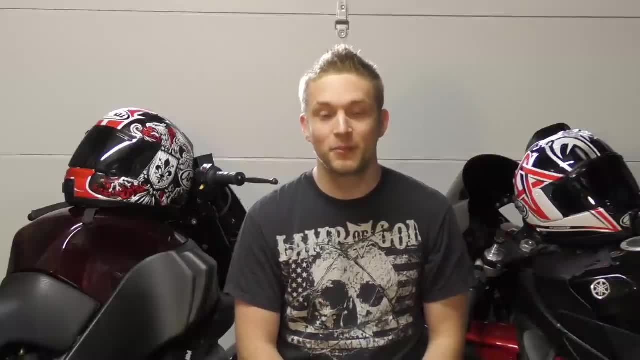 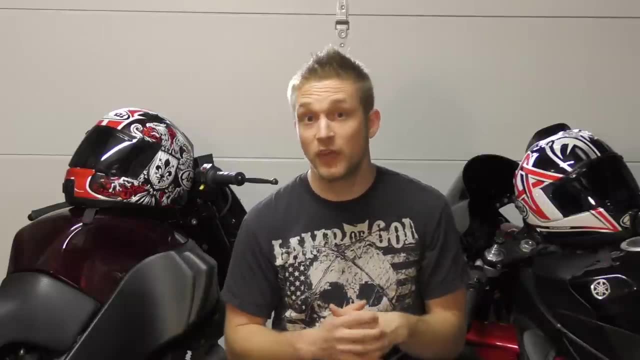 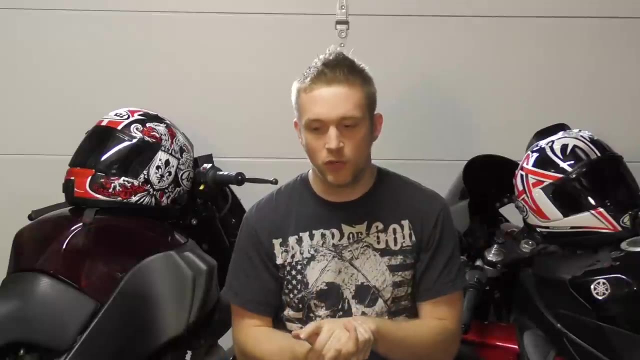 And then we had to get a ride back from, you know, back from downtown Portland, which sucked. That was a really lame ride home. So I had insurance at the time and I met my insurance adjuster down at their office- His name was Bart- and give him all the details, give him my spare key- you know all that stuff- and he explains to me how it's going to work. 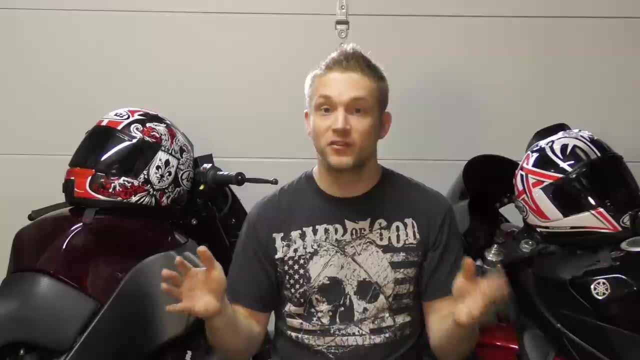 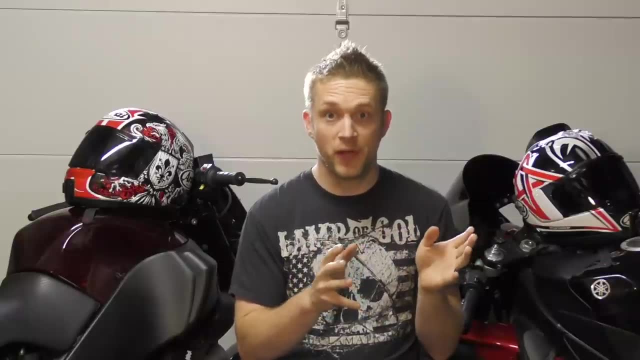 And then I wait the 30 days for Progressive to confirm that my bike is in fact gone for sure. I think I got three or four grand for it. It was a pretty mediocre amount. The only time I ever bought a bike from a shop was this experience. 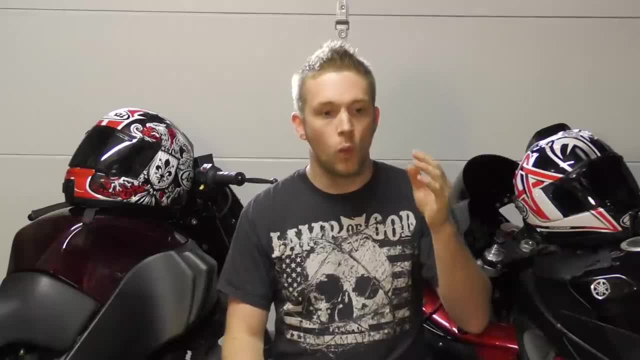 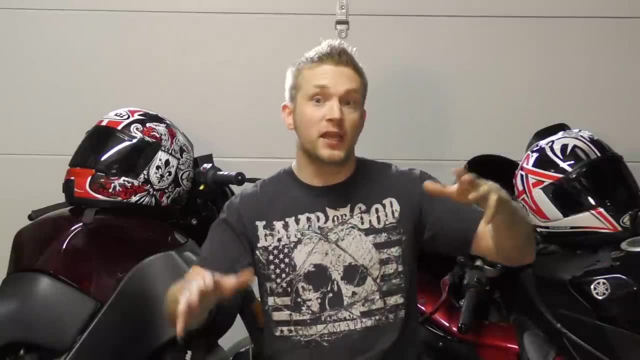 I walk into the dealership, They have this beautiful white 2009 R1.. It's 2010.. They're just getting ready to bring in the 2010 R1.. So they're looking to get rid of it, But it's like a floor model that they had done a bunch of customizations to and they were trying to push for. I don't know. 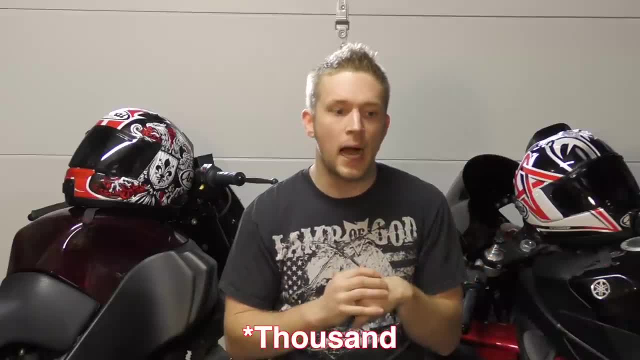 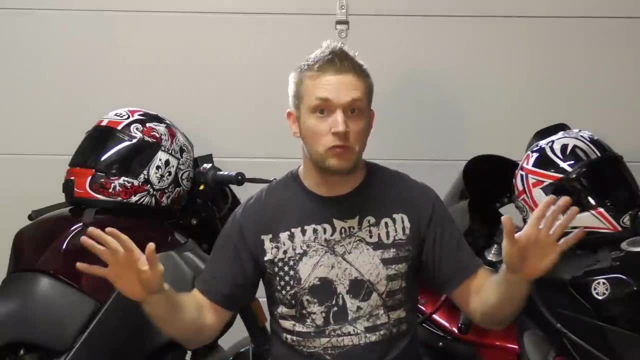 I think they were trying to sell it for like $1,700, $1,800., But they were going to sell it to me for like $1,200.. Which to me was great. Fine, Whatever. Brand new bike. 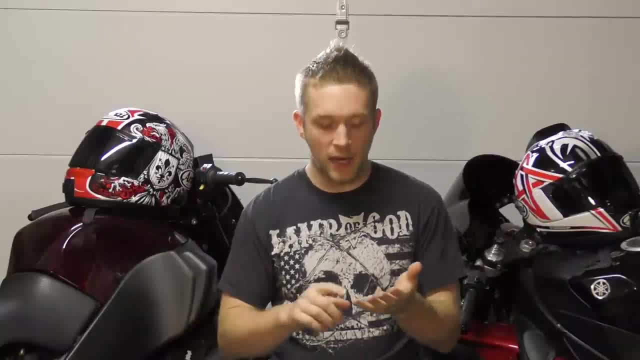 Right off the show floor. I was pretty stoked. I don't even remember all the accessories it had on it. It had, I think, a power commander, a different exhaust, different sprocket chain, whatever. A bunch of stuff. 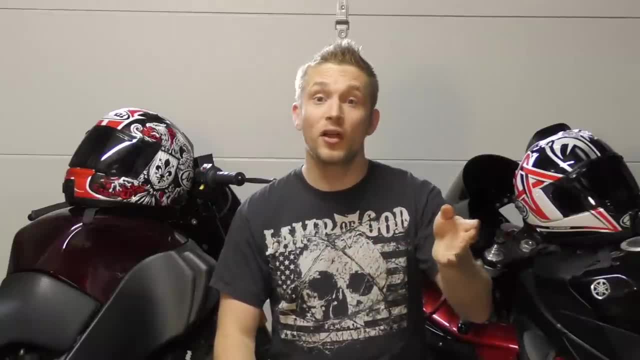 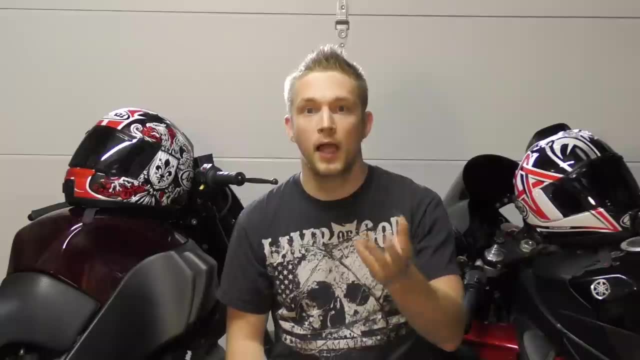 I don't remember really, because they didn't have the bike that long Spoiler warning. So I get the brand new bike and I start parking it right outside my bedroom window in a carport in my apartment. I wake up early on a Saturday morning to go to work. 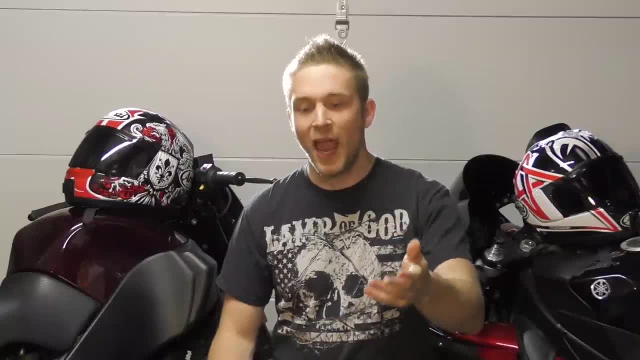 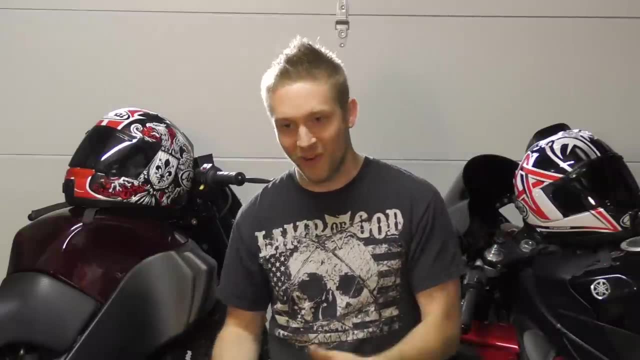 And as I walk out to my carport I look and my bike is fucking gone again And of course theft is the first thing on my mind again. So I call Progressive again And you know what I get? the exact same insurance adjuster Bart. 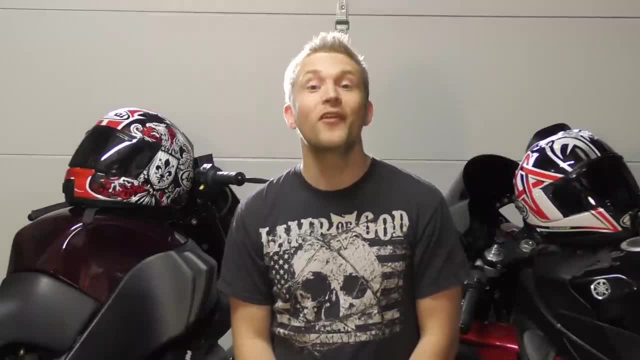 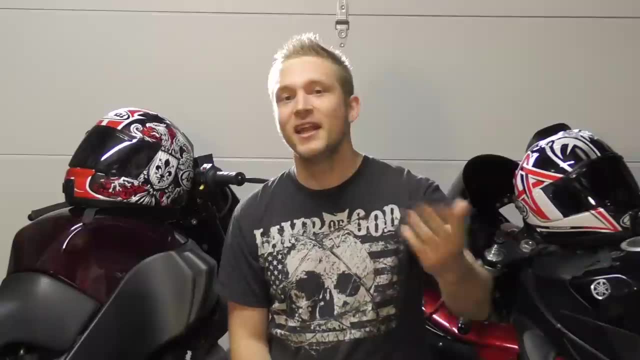 And this time Bart is less nice to me. He is less kind to me. He's actually more like irritated that I'm so fucking stupid to get my bike stolen again, Which in his defense, he's probably right. I definitely should have done something different. 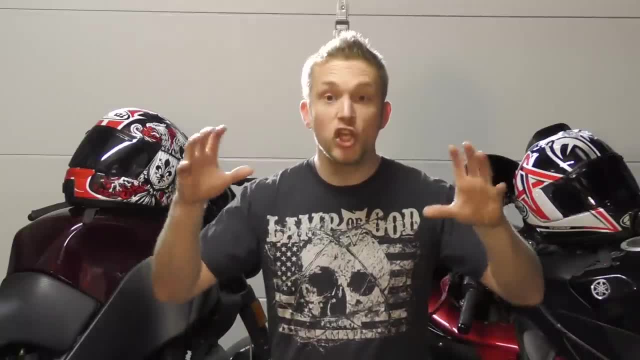 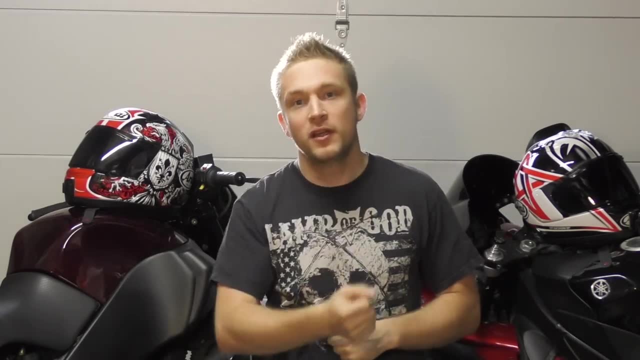 Since that point I haven't had a problem. Like I said, I grabbed a huge chain- These like bulldog 25, 30 pound chains And I strapped it through my frame at work and through my frame at home. 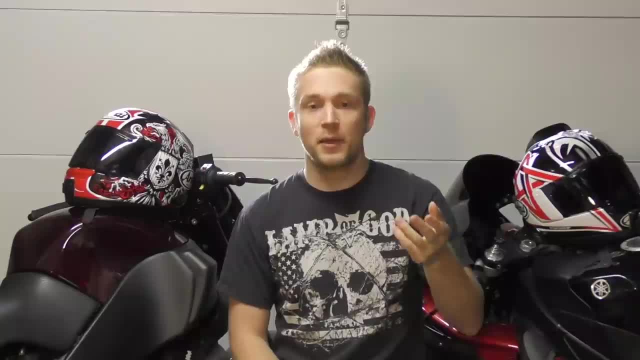 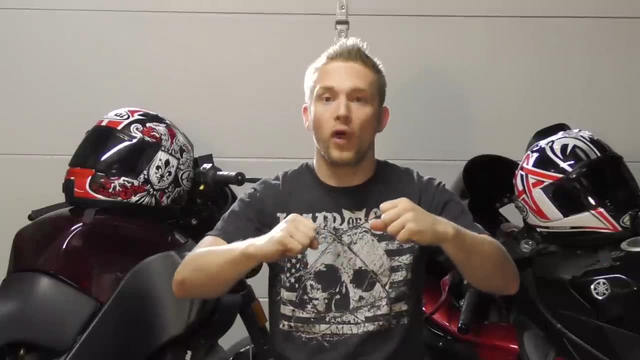 The chain actually led to another complication. So I was working retail at the time at a Best Buy down in the Portland area And I started to park up on the side where the bike locks were because there was a big metal pole I could strap it to. 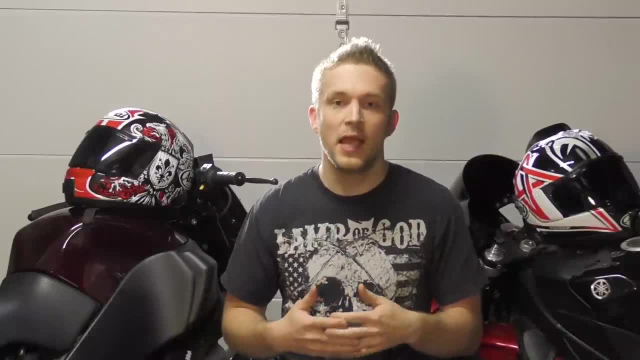 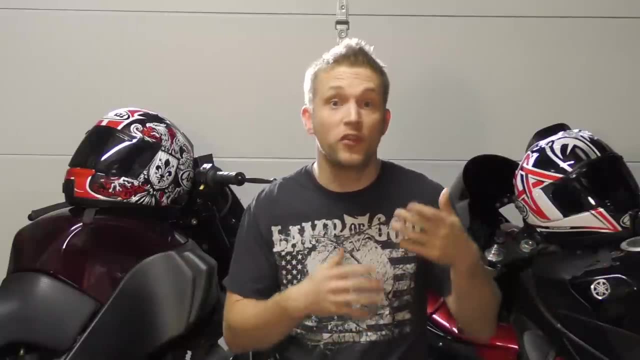 And that pissed off the security guards. So one of the security guards comes in and starts yelling at me, telling me I can't park there, Not really explaining why. I explained to him I've had a motorcycle stolen and that this is what I'm going to do. 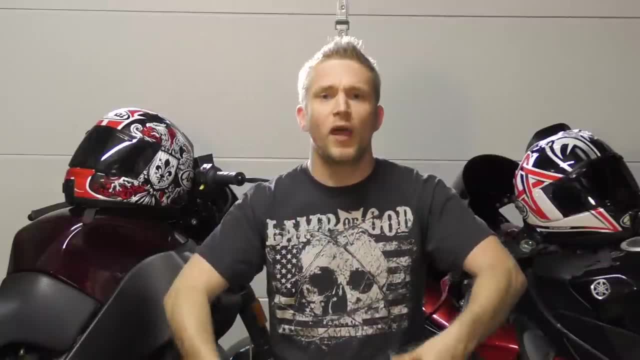 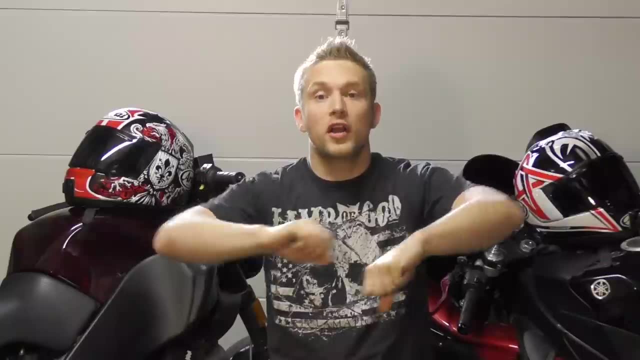 And this is the only place I can really strap it Because there's like the light poles. they had had huge like concrete things around it to protect them, So I couldn't really like the chain wasn't long enough for me to strap it around that. 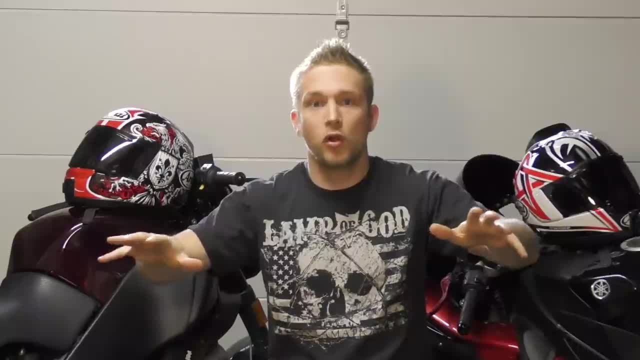 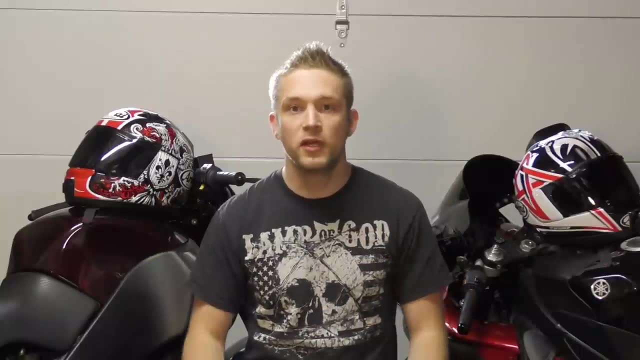 So this was the only place I could strap it to be anywhere close or anywhere visible. We more or less escalate to it. There's a screaming match in the store And he finally tells me that he's going to call and get the bike towed. 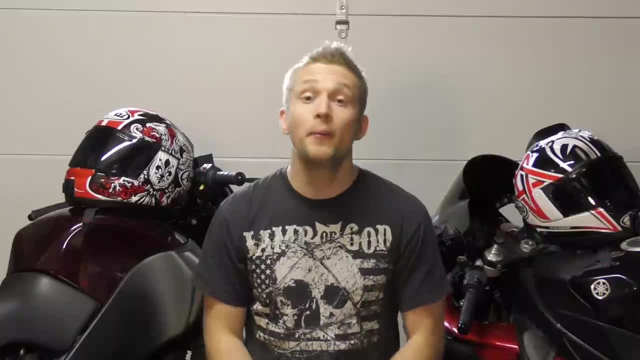 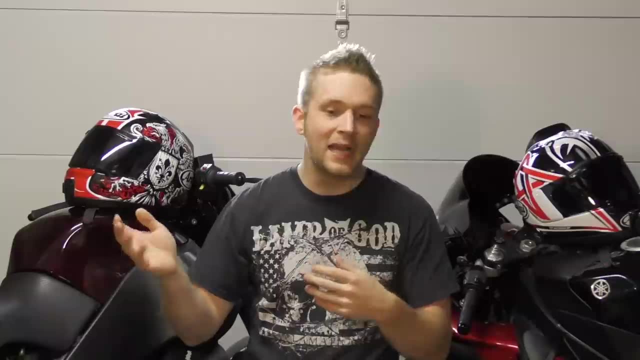 And I tell him to fucking good luck and try, because that chain is thick as shit. About a week later, a different security guard came in who was significantly nicer- I think he was like head of security or whatever- And he explained to me some reasons why they didn't want me to park my bike. 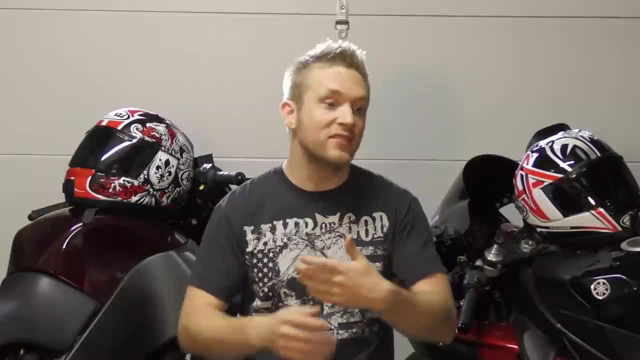 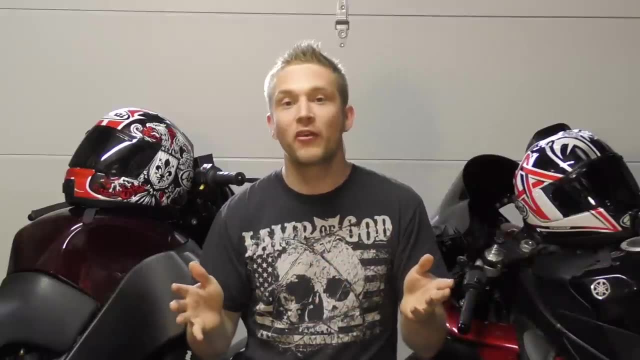 And in the end I basically just said, look, I'm going to keep doing it. And they said, as long as the general manager was okay with it, they were fine with it, which he definitely was. So that's pretty much how the story ended. 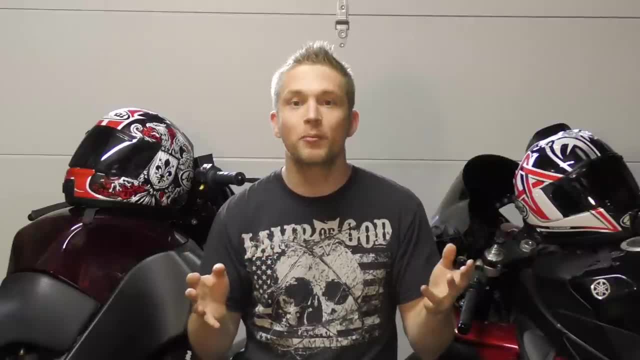 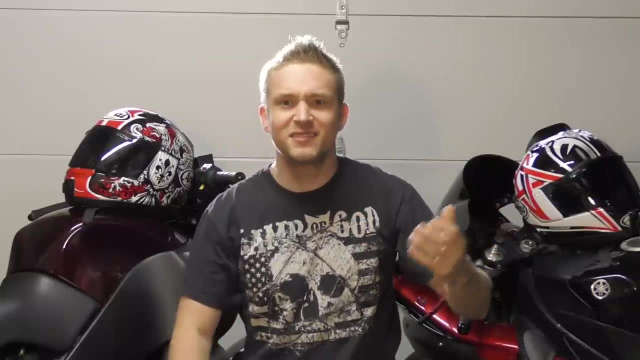 I kept walking there for about two years And never had a problem again And that was the first time I ever fought the power. I don't know, Is that racist? That's kind of like a Black Panther thing, I don't know. Anyway, I should probably cut that.